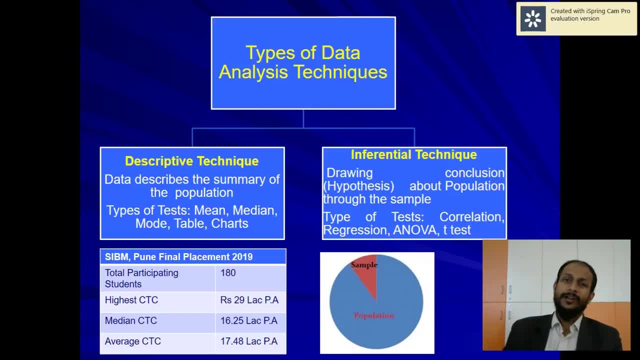 CTC is 17.25 lakhs per annum. So it is quite evident that what is the highest package, what is the average package, what is the median package? everything has been represented through the data that is available from the 180 students. Now, this is a typical example. 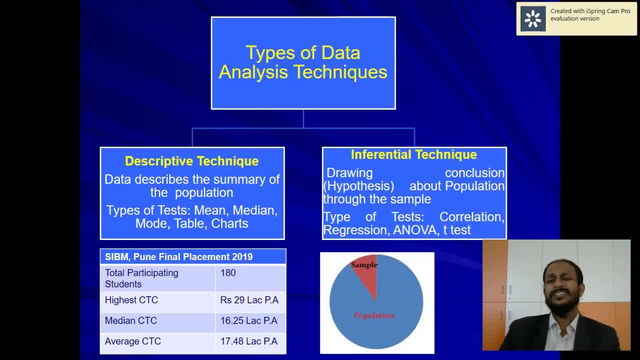 of a descriptive statistical technique. Here you can see that I have not taken any particular sample, but I have considered the entire data of the population, and I am talking about the population through the entire data that is available. Now this is what we call it as descriptive statistics. Now let us discuss about another. 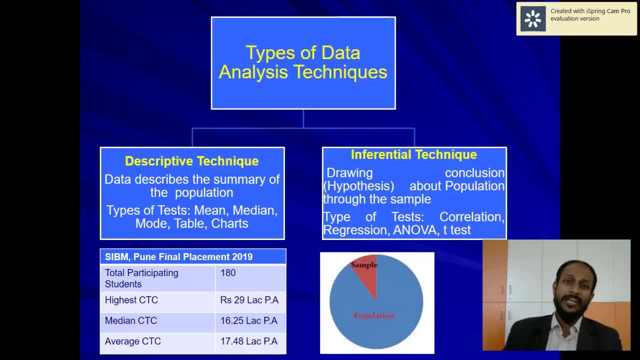 technique which comes under statistic, called inferential statistics. Now look at the word carefully, denote the word. they have used something called inference. That means I am actually inferring about something through something else Here. what do we do? we predict the characteristics of the population through the sample that is available. That is why we have used the 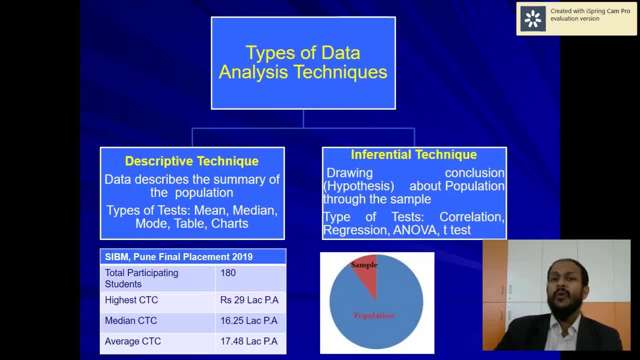 term called inferential statistics. So this is what we call it. Now let us discuss about the inferential statistics. so what i do is that i start predicting the population and i use something called hypothesis for this. so i take about a set of sample and i predict about the characteristics. 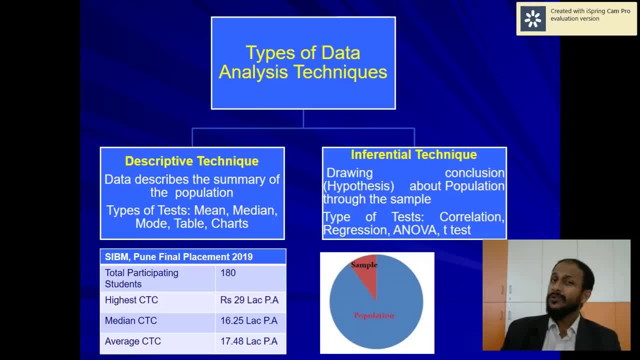 of the population say, for example, in 2021, it is expected that the legislative assembly is going to. the election is going to happen in tamilnad and almost let's say that there are, some say, 234 constituencies in tamilnad and i'm not sure which is the political party which is going. 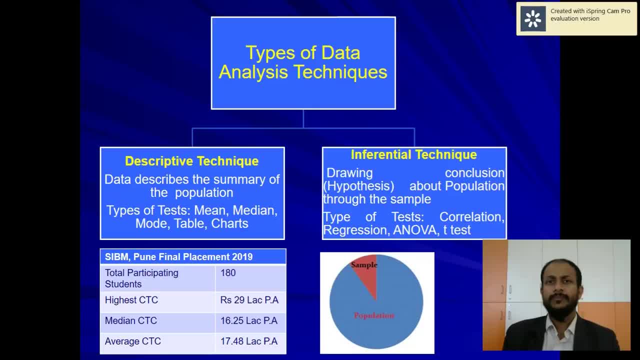 to come. it might be dmk, admk, congress or bjp. now, if at all, i wanted to know which political party is going to come to the power during 2021 mla election. the easy way is that i need not to check with each and every 5.8 crore voters in tamilnad. instead, i can take the constituencies start. 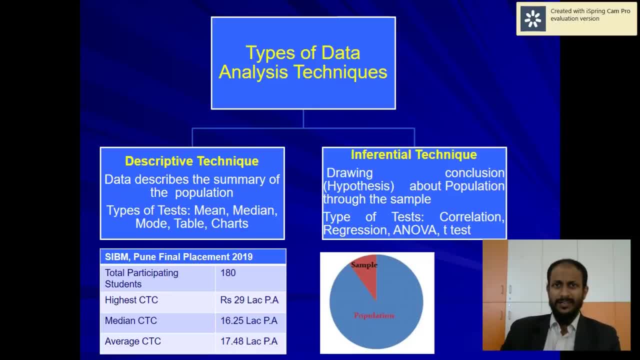 package. what is the median package? everything has been represented through the data that is available from the 180 students. Now, this is a typical example of a descriptive statistical technique. Here you can see that I have not taken any particular sample, but I have considered. 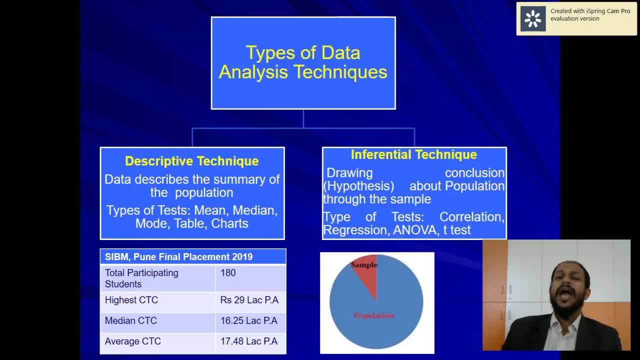 the entire data of the population, and I am talking about the population through the entire data that is available. Now this is what we call it as descriptive statistics. Now let us discuss about another technique which comes under statistic, called inferential statistics. Now look at the. 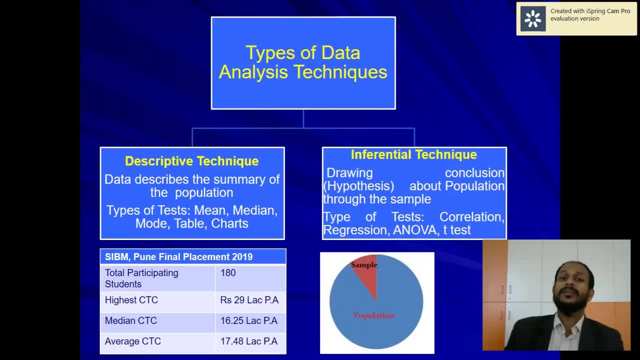 word. Carefully denote the word. They have used something called inference. That means I am actually inferring about something through something else. Here, what do we do? We predict the characteristics of the population through the sample that is available. That is why we have 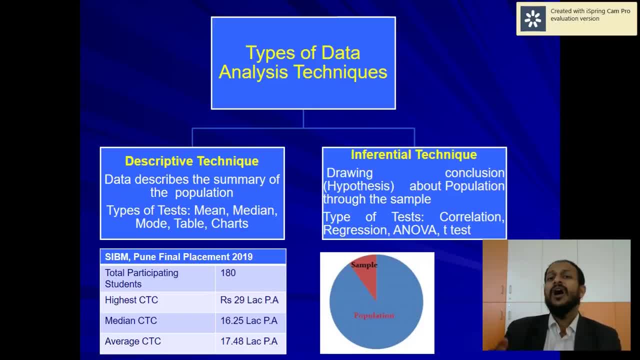 used the word inferential statistics. Now let us discuss about another technique which comes under the term inferential statistics. So what I do is that I start predicting the population and I use something called hypothesis for this. So I take about a set of sample and I predict about the 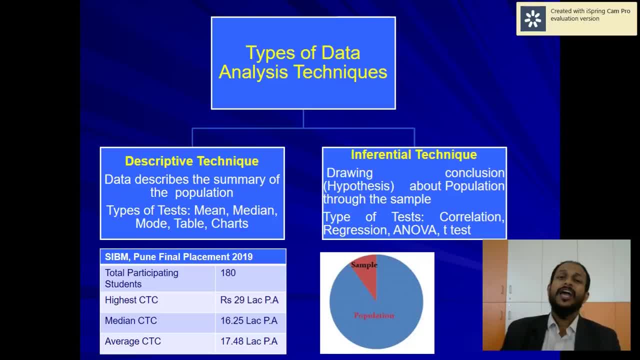 characteristics of the population. Say, for example, in 2021 it is expected that the legislative assembly is going to have, election is going to happen in Tamil Nadu and almost let us say that there are, some say, 234 constituencies in Tamil Nadu and I am not sure which is the political party. 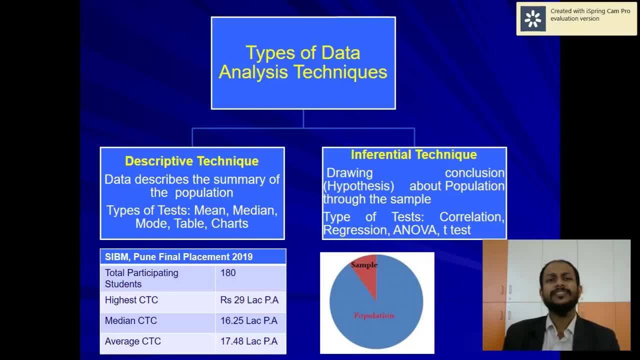 which is going to come. It might be DMK, ADMK, Congress or BJP. Now, if at all, I wanted to know which political party is going to come to the power during 2021 MLA election. The easy way is that I need not to check with each and every 5.8 crore voters in Tamil Nadu. Instead, 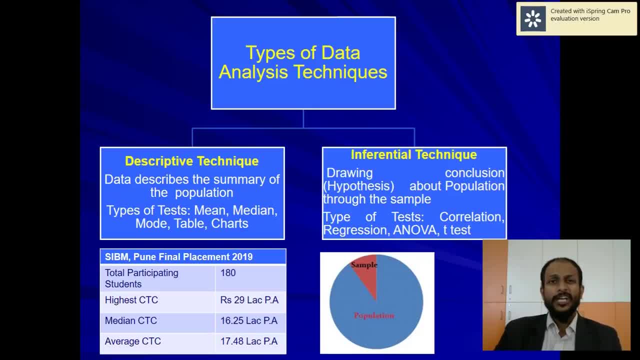 I can take the constituencies, start checking with 100 people each, and 100 into 234.. This is the number of people that I have surveyed and from that survey, I am predicting that who is going to win this 2021 MLA election. Now, this is what we call it as inferential statistics. That means: 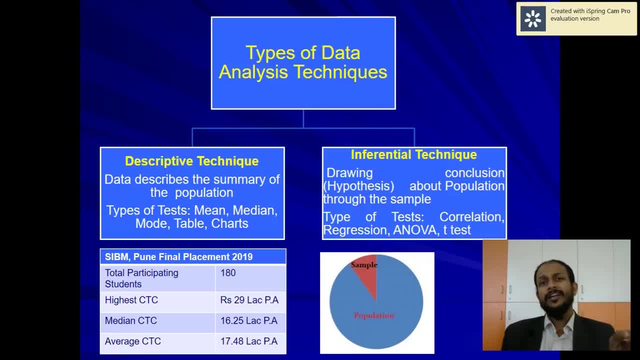 checking with 100 people each, and 100 into 234. this is the number of people that i have surveyed, and from that survey, i'm predicting that who is going to win this 2021 mla election? now, this is what we call it as inferential statistics. that means, instead of i conducting a survey among 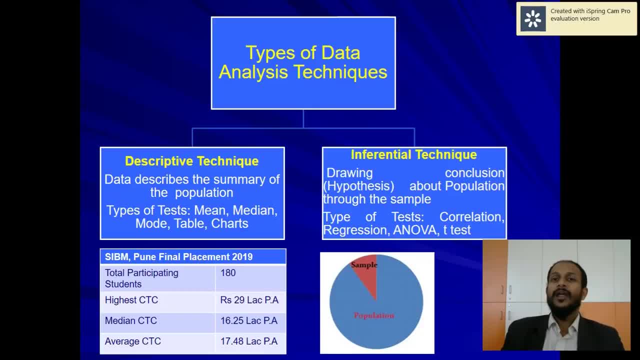 5.8 crore people in tamilnad. i have taken a shortcut. what i have done? i have taken 100 people each from 234 constituencies, which comes something around 23 400 samples and from there i'm predicting that who could be the possible winner in the upcoming 2021 mla election, and i'm 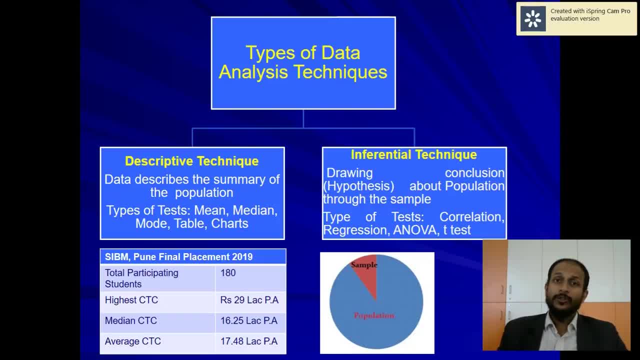 telling this with 95 percent confidence, with five percent margin of error. now look at the difference in the statement, guys. when i have told you about the descriptive statistics, i did not use anything like confidence interval margin of error. now, this normally we will not use when it comes to descriptive statistics, when it comes to 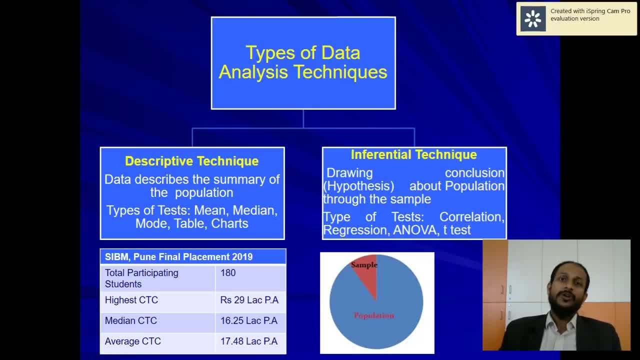 inferential statistics. i am not hundred percent sure. i might be 90 to 95 percent sure, and i also have some kind of tolerance of five to ten percent, which i call it as margin of error in statistical terms. now, this is the kind of understanding that we need to have when it. 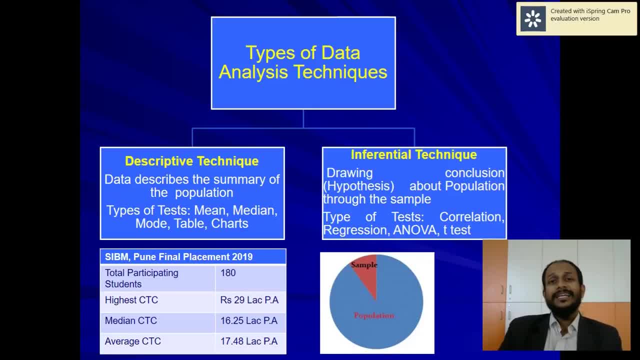 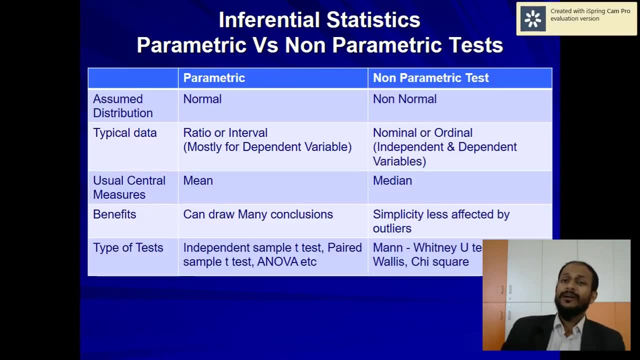 comes to the inferential statistics. now let us get deep into the inferential statistics because most of the time we will be doing many type of analysis under the category of inferential statistics so that we can prove or disprove our hypothesis. now, when it comes to inferential, 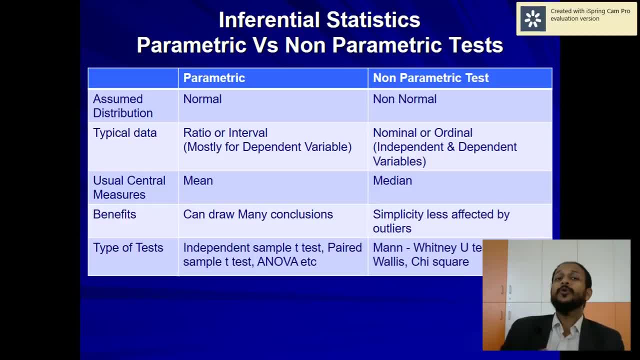 statistics. we can classify them into two broad categories. one is that parametric test and the other one is non-parametric test. what is meant by parametric test? make it simple: parametric test or those tests where you have some assumption about the population? i hope already have told you. 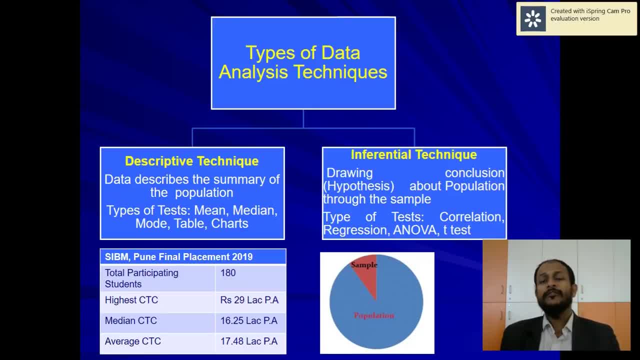 instead of I conducting a survey among 5.8 crore people in Tamil Nadu, I have taken a shortcut. What I have done, I have taken 100 people each from 234 constituencies, which comes something around 23,400 samples, and from there I am predicting that who could be the possible? 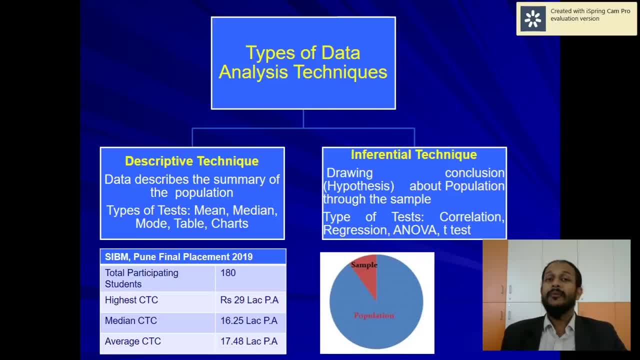 winner in the upcoming 2021 MLA election, and I am telling this with 95% confidence, with 5% margin of error. Now look at the difference in the statement, guys. When I have told you about the descriptive statistics, I did not use anything like confidence. 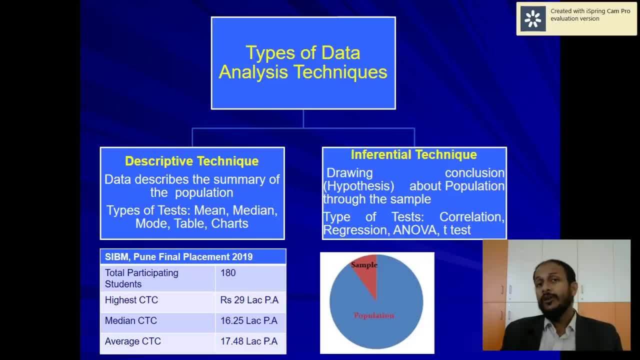 interval margin of error. Now, this normally we will not use when it comes to descriptive statistics, When it comes to inferential statistics, I am not 100% sure. I might be 90 to 95% sure, and I also have some kind of tolerance of 5 to 10%, which I call it as margin of error. 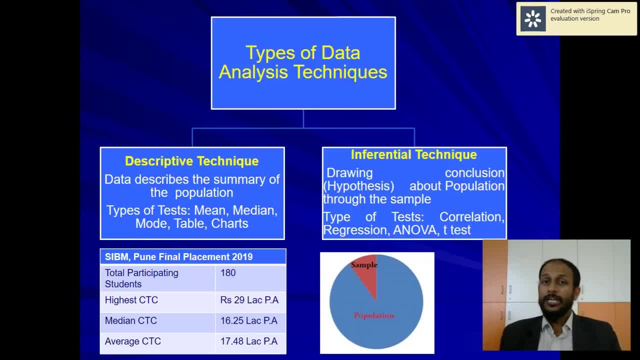 in statistical terms. Now, this is the kind of understanding that we need to have when it comes to the inferential statistics. Now let us get deep into the inferential statistics, because most of the time, we will be doing many type of analysis under the category of inferential. 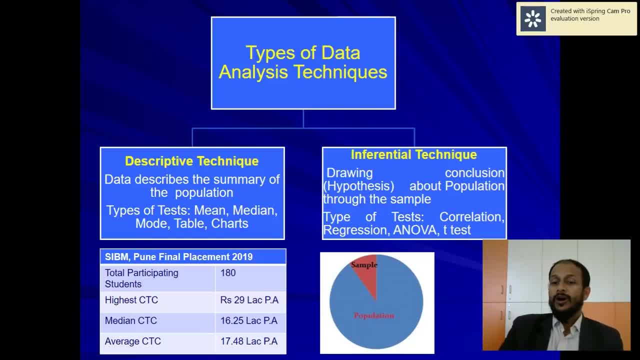 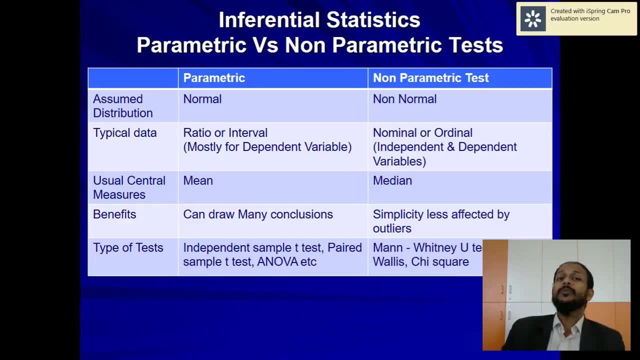 statistics so that we can prove or disprove our hypothesis. Now, when it comes to inferential statistics, we can classify them into two broad categories. One is that parametric test, and the other one is non-parametric test. What is meant by parametric test? It is a 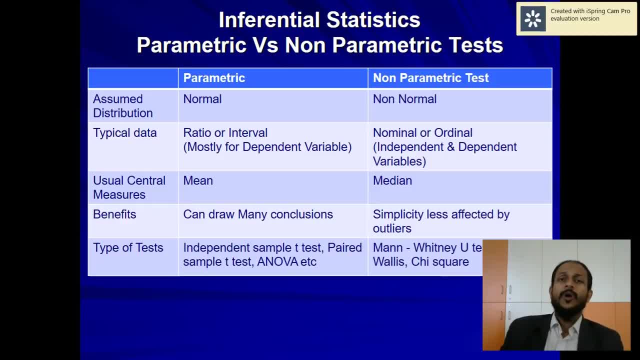 parameter test or a clinical test where you can take a sample of a particular�� or random event. from the sample is here, somelle étant same as a meplanter test, where you can also create느 as a machine would make it simple. parametric test, or those tests where 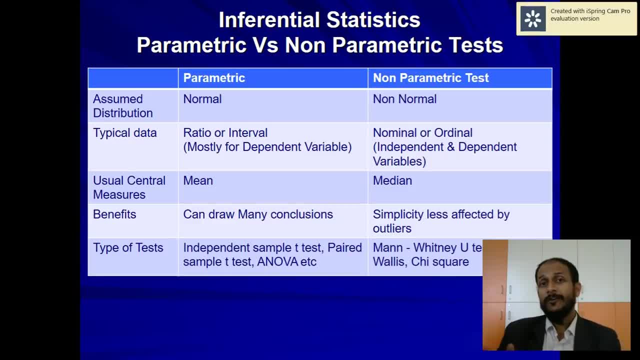 you have some assumptions about the population. Now, I have told you already that inference statistics is all about you predicting the characteristics of the population to the sample. Now, parametric test is something you have some assumption about- the population from where you are drawing the sample, And this assumption is something related with normality. 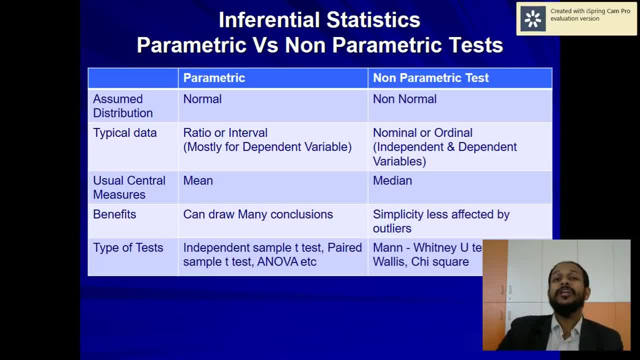 where you assume that the probability of example being a non-parametric test would be different than that a weak non-parametric test will be the highest. So first you have an assumption: The population that you are drawing is a normal data. it is a normal population. 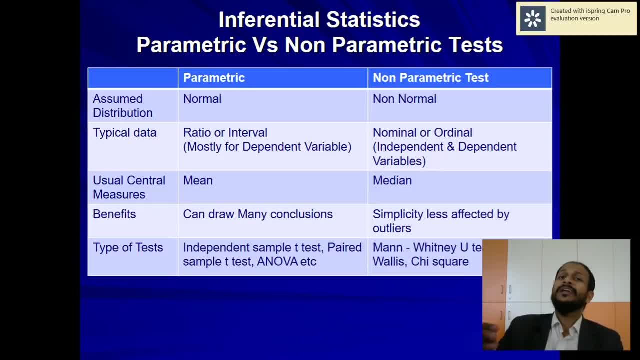 that inferential statistics is all about you predicting the characteristics of the population through the sample. now, this parametric test is something you have some assumption about the population from where you are drawing the sample, and this assumption is something related with normality, where you assume that the population that 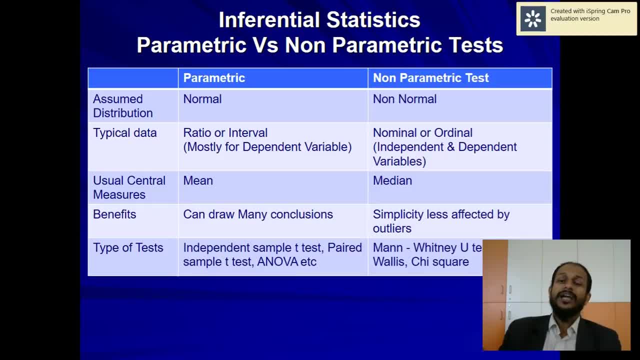 you are drawing is a normal data, it is a normal population. now, when you have this set of assumption, thinking that the population from where i am drawing the sample is normal and my sample data is also normal, that time i have a choice to use parametric test. now, when these assumptions 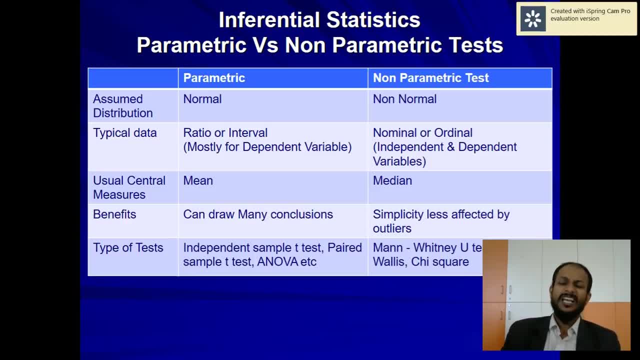 are not been met. that time i will be using non-parametric test, like dollars. we have classified the test into two broad categories, depending upon the distribution right. let us discuss it one by one so that let us get some idea on what test that we have to use for our analysis. now, when it comes to the parametric test, as i have already told, 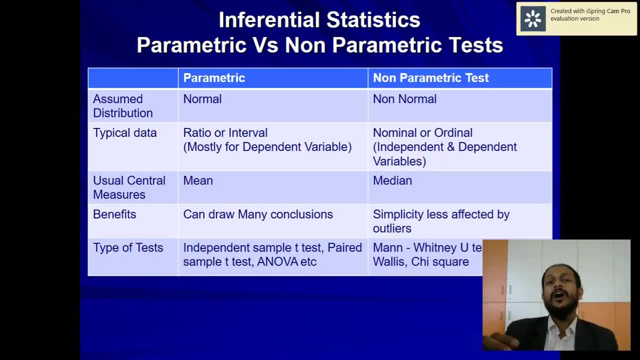 you that parametric test is usually upright for something which is normal, but when it comes to non-parametric test, it is not necessary that it should be normal. so it is a distribution-free test. so the first difference is: parametric test, the data is normal. when it comes to non-parametric test, the data is not normal. and the second one is that when it 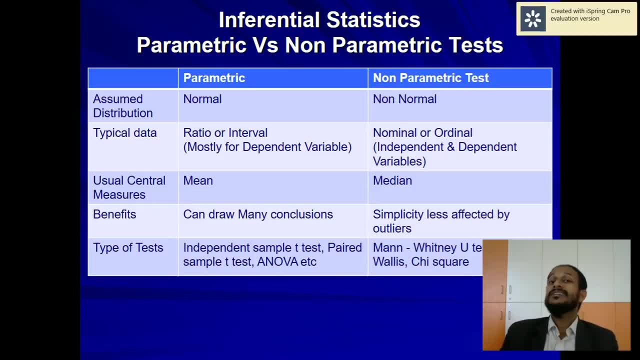 comes to the type of data. the type of data in parametric test is continuous. it could be either ratio or interval and mostly it is for the dependent variable, especially when we discuss about the techniques like ANOVA or student tick test. we talk only about the different. 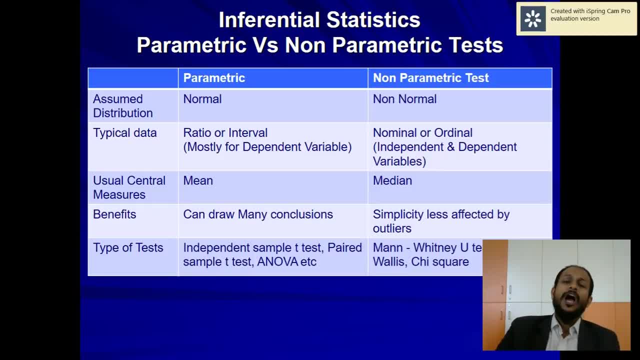 dependent variable when it comes to the continuous scale. of course, it is also applicable for independent variable also in case, if at all, we are planning to use something like regression or correlation right. second one is that non-parametric test in non-parametric test, the typical set of 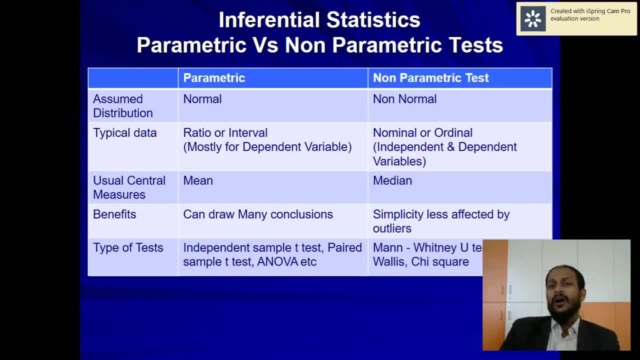 data. it is either nominal or ordinal, so it is applicable for both independent as well as for dependent variable. the second, the third one, is that when it comes to these central measures, usually we will be able to use something called mean for the parametric test, whereas when it comes to the non-parametric test, because the data that we have obtained is, 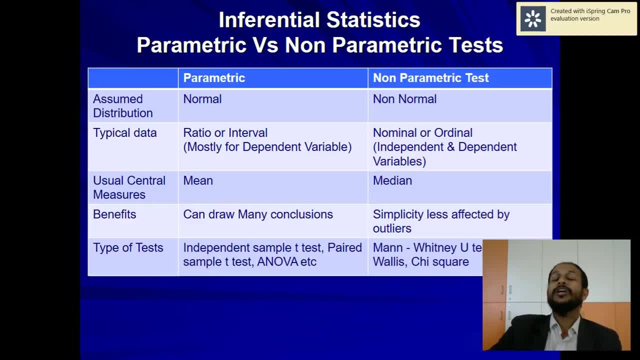 Now, when you have this set of assumption, thinking that the population from where I am drawing the sample is normal and my sample data is also normal, that time I have a choice to use parametric test. Now, when these assumptions are not been met, that time I will be using non-parametric test. 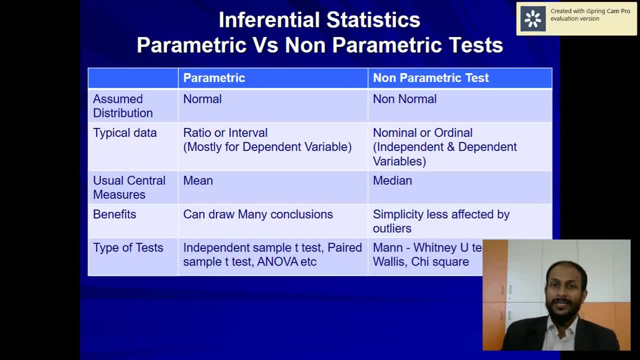 Like this: we have classified the test into two broad categories, depending upon the distribution. Let us discuss it one by one so that let us get some idea on what test that we have to use for our analysis. Now, when it comes to the parametric test, as I have already told you, that parametric test 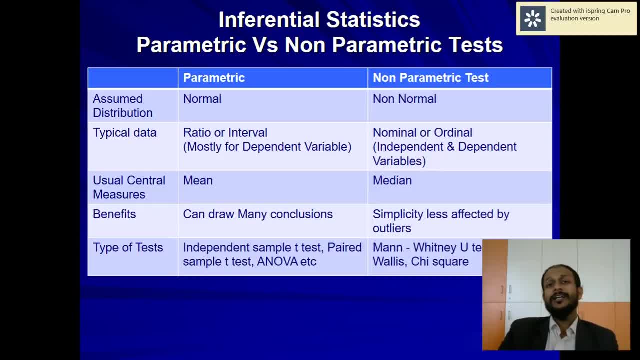 is usually applied for something which is normal. But when it comes to non-parametric test, it is not necessary that it should be normal. so it is a distribution free test. So the first difference is: parametric test: The data is normal. when it comes to non-parametric test, the data is not normal. 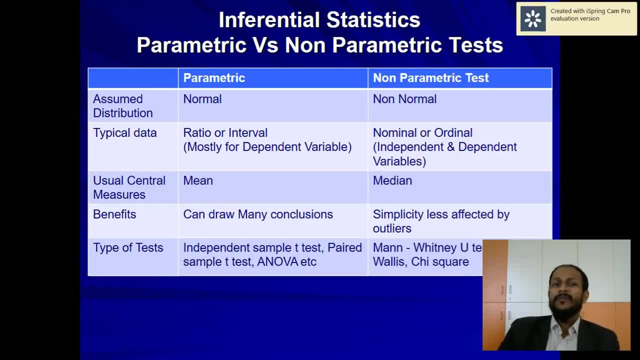 And the second one is that, when it comes to the type of data, the type of data in parametric test is continuous. It could be either ratio or interval and mostly it is for the dependent variable, especially when we discuss about the techniques like ANOVA or student tick test. 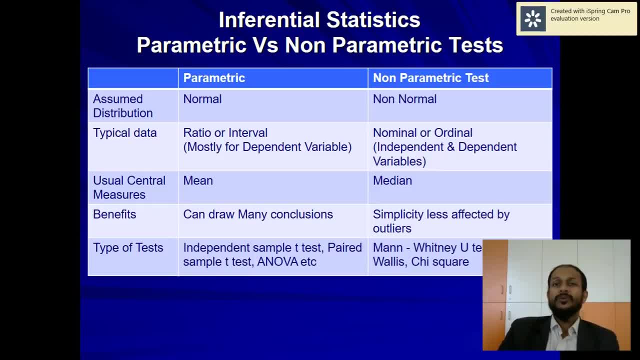 We talk only about the different dependent variable when it comes to the continuous scale. Of course, it is also applicable for independent test. So it is a distribution free test. It is a dependent variable also in case, if at all, we are planning to use something like. 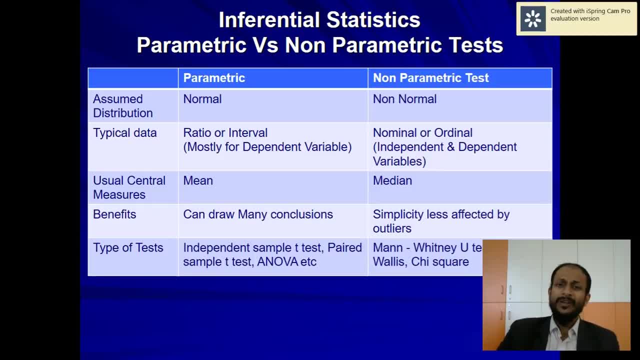 regression or correlation. Second one is that non-parametric test, In non-parametric test, the typical set of data. it is either nominal or ordinal, So it is applicable for both independent as well as for dependent variable. The third one is that, when it comes to the central measures, usually we will be able to: 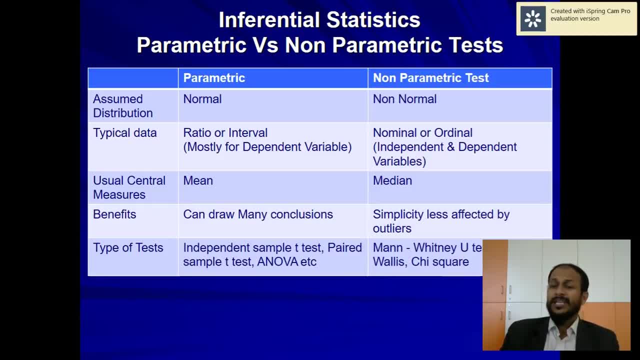 use something called mean for the parametric test, Whereas when it comes to the non-parametric test, because the data that we have obtained is only in the form of either nominal or ordinal, we can use a technique like median. We cannot use techniques like mean, like in terms of parametric test. 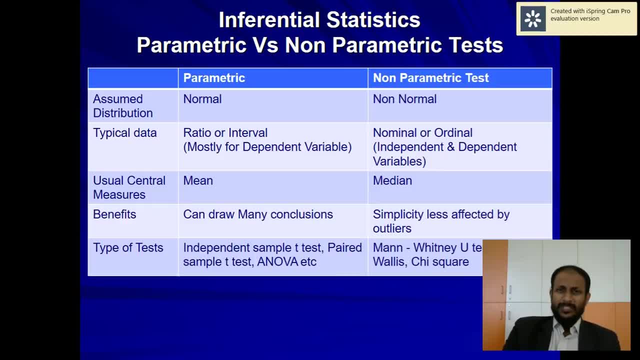 The other one is that we can draw many conclusions based on parametric test, but we cannot have so many conclusions based on non-parametric test. We can also have one more difference, Like The sample size. parametric test require a bigger sample size. 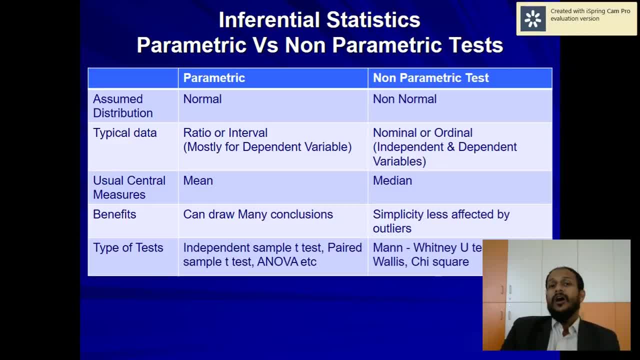 only in the form of either nominal or ordinal. we can use a technique like median. we cannot use techniques like mean, like in terms of parametric test. the other one is that we can draw many conclusions based on parametric test, but we cannot have so many conclusions based on. 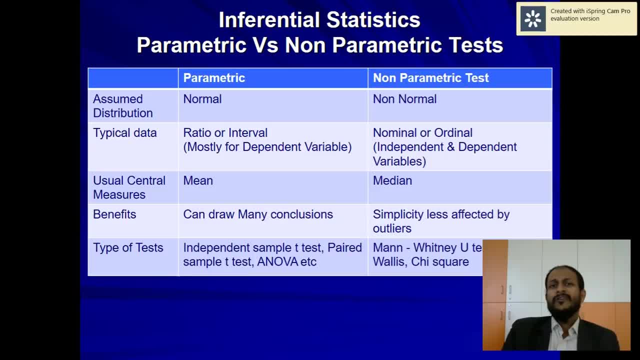 non-parametric test. we can also have one more difference, like when it comes to non-parametric test, when it comes to the sample size. parametric test require a bigger sample size. when it comes to non-parametric test, you don't need to have that much big sample size. it might give you a good. 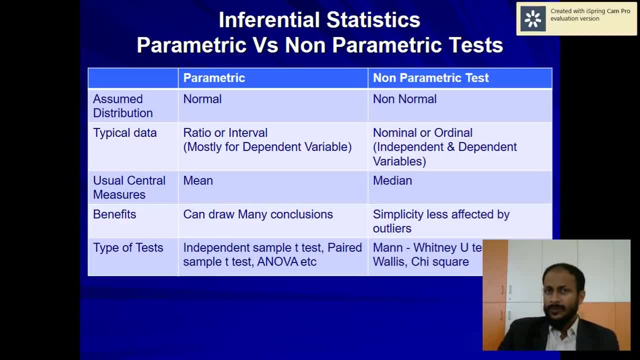 result when it comes to a small sample size also. the last one is: which is the most important in today's session is that, when it comes to the different type of test, I can use tests like independent sample t-test, pad sample t-test, so on and so forth, other type of test in parametric test. 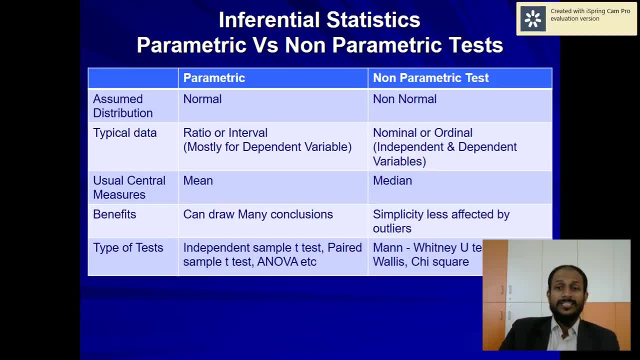 non-parametric test like Mann Whitney's use test, Kruskal Valley's test, chi-square test. so these are all the different kinds of non-parametric test that I can use for my analysis. so these are the main two broad classifications that we need to understand when it comes to whether we have to use this. 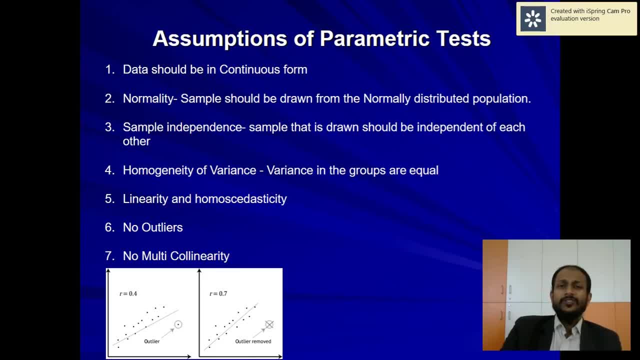 parametric test and non-parametric test. now let us also discuss about some of the assumptions of parametric tests, so that let us give some kind of clear idea. already I have told you about the parametric test and non-parametric test. let us discuss about the assumptions one by one, so that 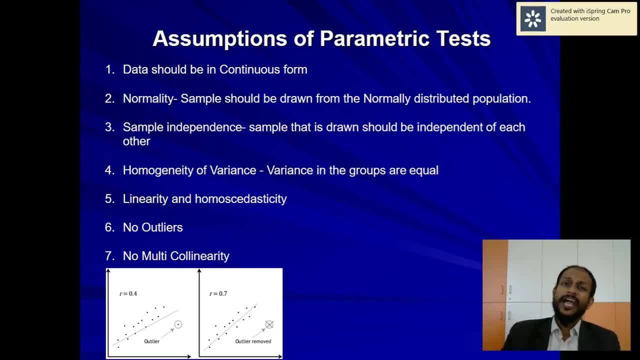 and we will be very clear that which type of test that I need to use for my analysis technique. the number one assumption, the most important assumption, is that the data that I am having about the sample or about the population, it should be in continuous form. that means either it should be interval or it. 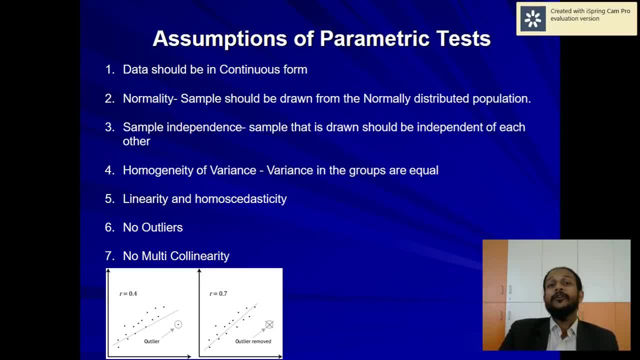 should become both independent and dependent variable as categorical variable when it comes to the parametric test. this should be the first and foremost assumption for the parametric test, no matter whether you are using correlation regression student test right. the second important assumption is that about normality. that means the sample data that I am drawing. 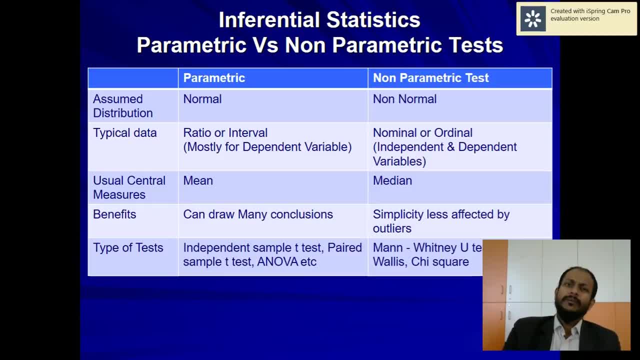 When it comes to non-parametric test, you don't need to have that much big sample size. It might give you a good result when it comes to a small sample size also. The last one is: which is the most important in today's session is that, when it comes to 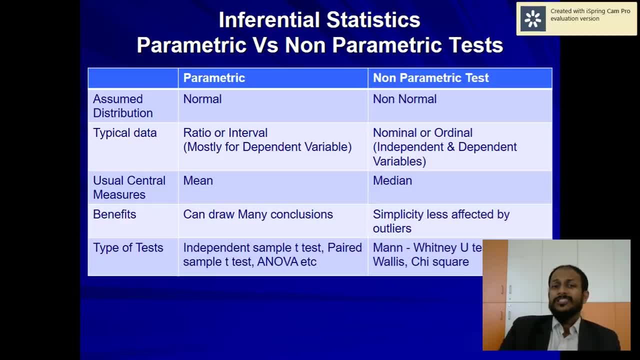 the different type of test. I can use tests like independent sample t-test, pad sample t-test, so on and so forth, Other type of test in parametric test And the equivalent non-parametric test. So I can use parametric test like Mann, Whitney's use test, Kruskal Valley's test, chi square. 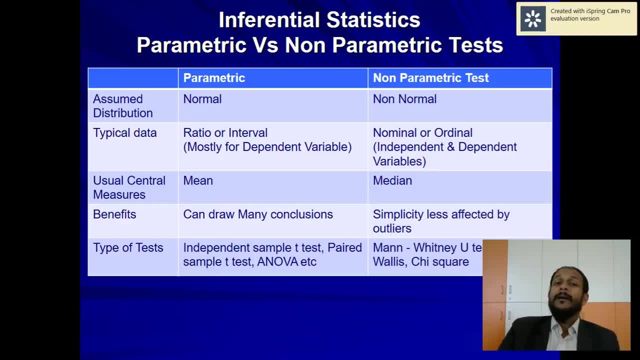 test. So these are all the different kinds of non-parametric test that I can use for my analysis. So these are the main two broad classifications that we need to understand when it comes to whether we have to use this parametric test and non-parametric test. 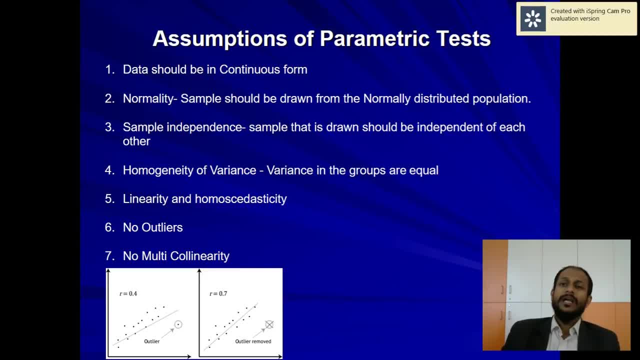 Now let us also discuss about some of the assumptions of parametric test, So that let us give some kind of clear idea Already. I have told you about the difference between parametric test and non-parametric test. Let us discuss about the assumptions one by one, so that we will be very clear that which 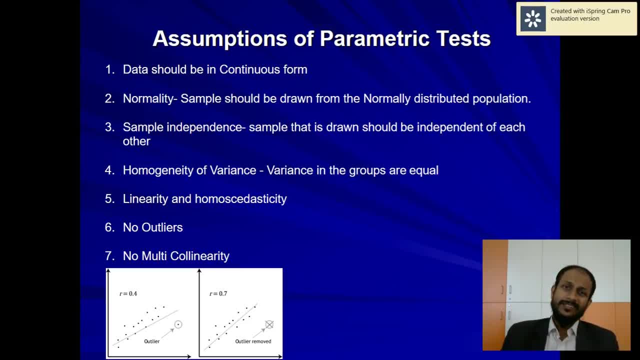 type of test that I need to use for my analysis technique. The number one assumption, the most important assumption, is that the data that I am having about the sample or about the population, it should be in continuous form. That means either it should be interval or it should be in the form of ratio. 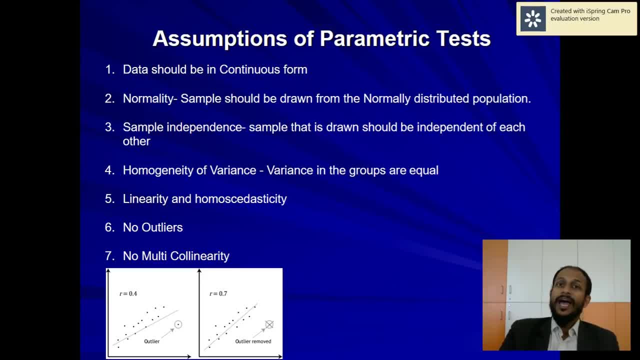 I can't have Both independent and dependent variable as categorical variable when it comes to the parametric test. This should be the first and foremost assumption for the parametric test, No matter whether you are using correlation regression student test. The second important assumption is that about normality. 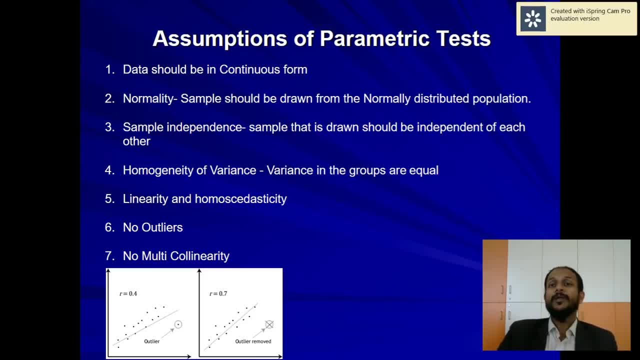 That means the sample data that I am drawing from the population. the population should be normally distributed. Now, what does mean by normality? Make it simple: normality is about the distribution of the data, and this distribution of the data is in such a way that most of the data is collected around the mean and very few data. 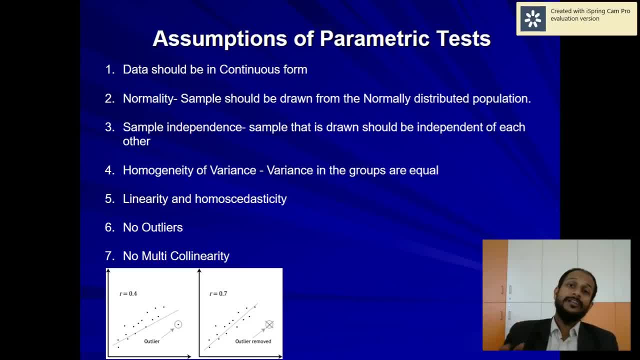 from the population. the population should be normally distributed. now, what does meant by make it simple? normality is about the distribution of the data, and this distribution of the data is in such a way that most of the data is collected around the mean and very few datas would be falling. 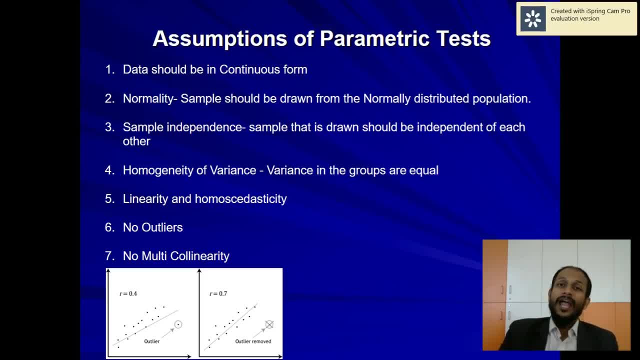 on the either sides. say, for example, if I am collecting your height and the height of the participants are ranging from 5 feet to 6 feet and the average of the height is almost 5.4, that is, 5 inches. the normality says that most of the data would be cluttered around. the mean very few people. 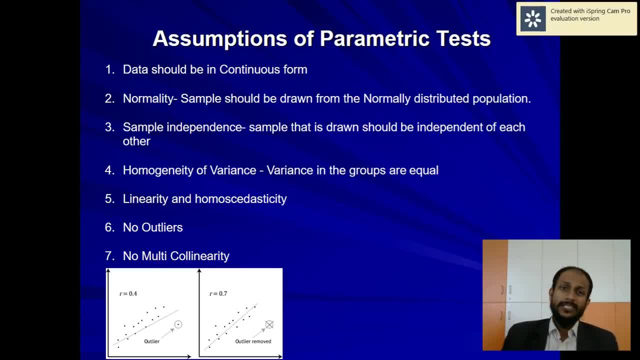 would be of 5 feet and very few people would be of 6 feet. now this is what we call it as normality in simple terms. now how do I check the normality of the data further? we have several tests. we have Shapiro Wilcox test and we have KS test. we do also have another test like I mean skewness and 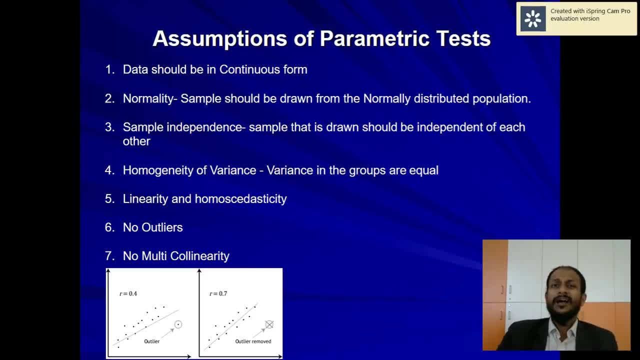 others. all these tests we can use and we can find out the data that they have collected is normal or not, but the best test that we can always recommend is that the Shapiro Wilcox test. now the third assumption is the sample that I am drawing. is it independent or not? I don't think so. uh, that. 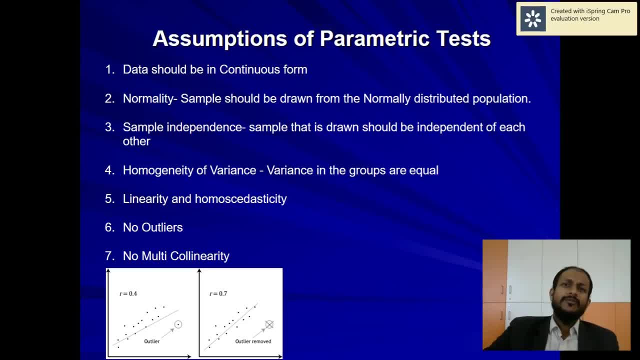 is something that needs to be explained, because it says that whenever I am drawing a sample from the population, the draw what I am making. it should be independent of the another draw right. it should be the third assumption. the fourth assumption is all about the homogeneity of 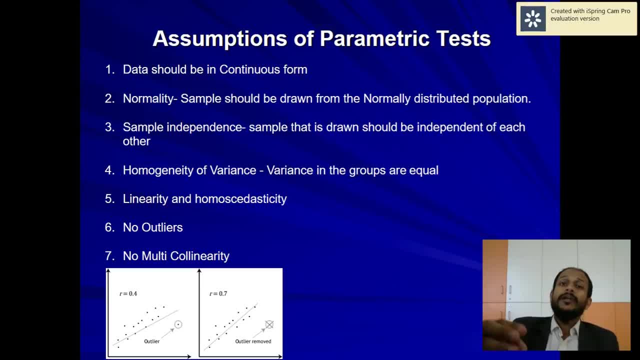 variance. that means the variance of the dependent variable across the independent variable. it should be equal. that means the standard deviation of the dependent variable, the standard deviation of the dependent variable which is present across two or three groups of independent variable. it should be equal. now, this is something it is. 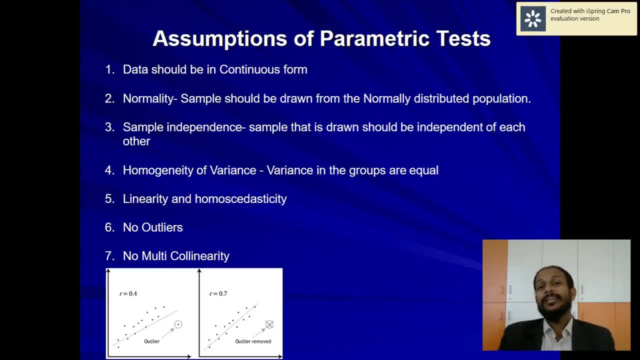 would be falling on the either sides. Say, for example, if I am collecting your height and the height of the participants are ranging from 5 feet to 6 feet and the average of the height is almost 5.4.. That is 5 feet 4 inches. 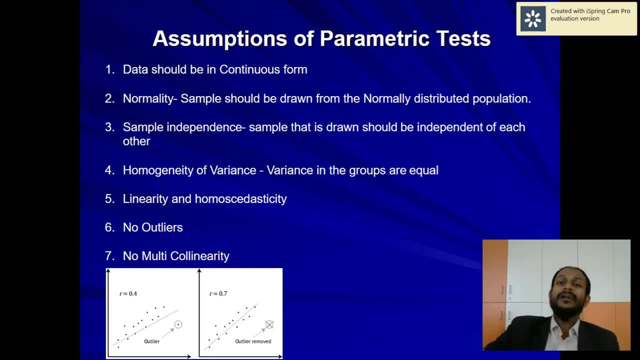 The normality says that most of the data would be collected around the mean. Very few people would be of 5 feet and very few people would be of 6 feet. Now this is what we call it as normality, in simple terms. Now, how do I check the normality of the data? 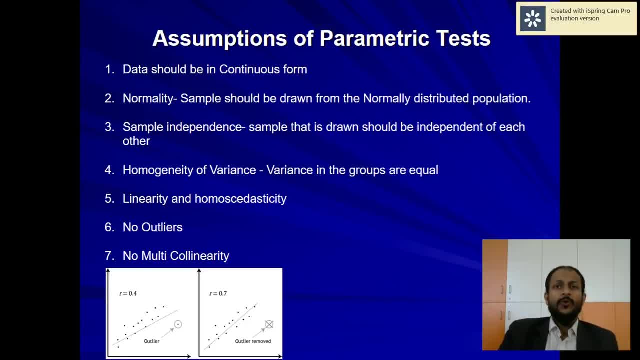 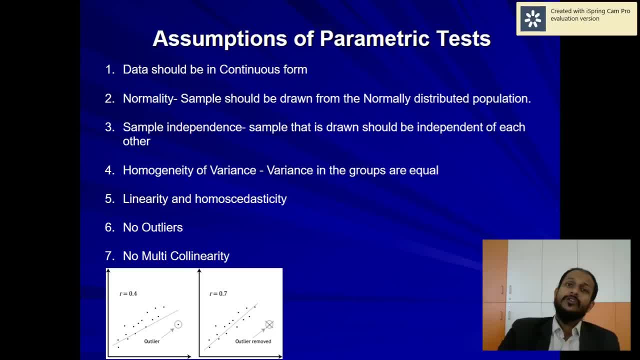 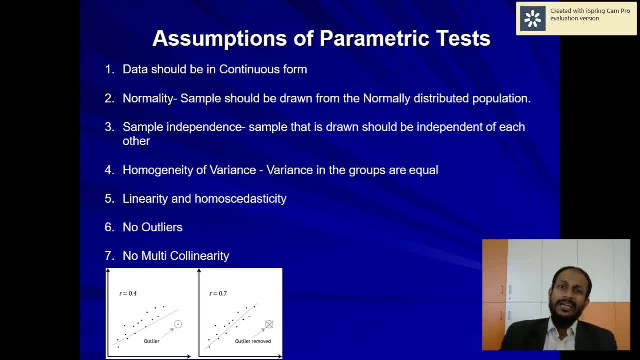 The third assumption is: the sample that I am drawing. is it independent or not? I don't think so. That is something that needs to be explained, because it says that whenever I am drawing a sample from the population that draw what I'm making, it should be independent of the 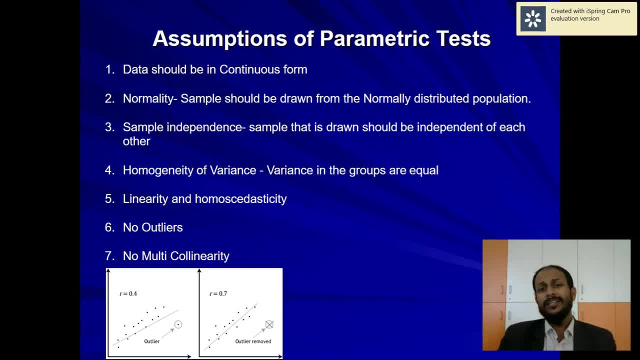 other draw right. this should be the third assumption. the fourth assumption is all about the homogeneity of variance. that means the variance of the dependent variable across the independent variable. it should be equal. that means the standard deviation of the dependent variable, the standard deviation of the 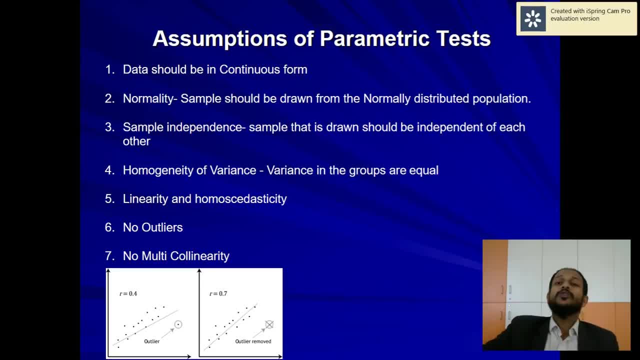 dependent variable which is present across two or three groups of independent variable. it should be equal. now, this is something it is related with, i mean anova, student t test, that we can explain it when you are explaining on the topic of anova or student t test, right, and when it comes to testing, 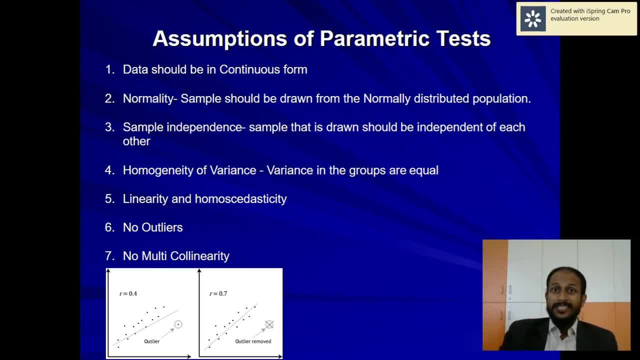 with I mean ANOVA, student t-test- that we can explain it when you are explaining on the topic of ANOVA or student t-test, right? and when it comes to testing of this type of assumption, usually use a test like Levene's test. so whenever the p-value is, we have some kind of critical and 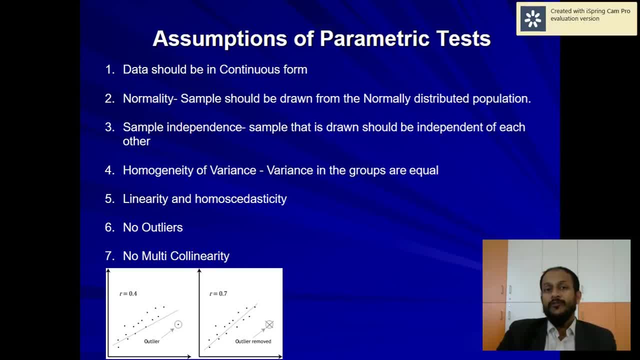 a cut-off point beyond which we fulfill the assumption of this type of test, under which we reject it. right. and the fourth type of assumption is all about the sorry. fifth one is all about linearity and homoscedasticity. so now this homoscedasticity and homogeneity. 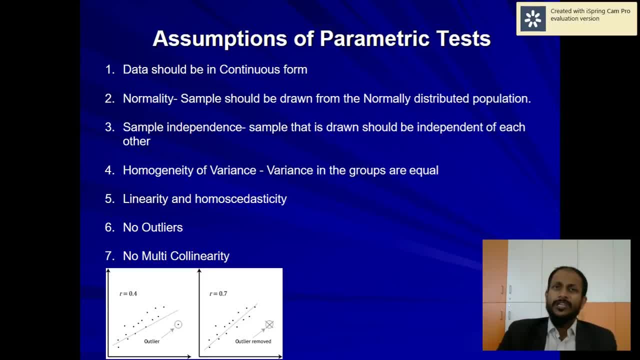 of variance is almost of same type. we use the word homogeneity of variance when it comes to ANOVA and student t-test, and we use the term homoscedasticity when it comes to the regression part. linearity is all about how the variables are linearly related. if at 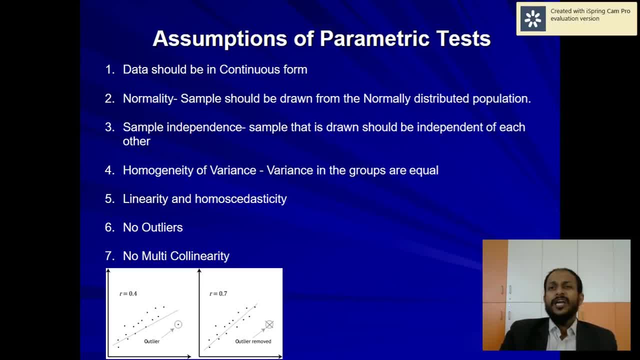 all I say about height and weight are related with each other. the linearity is all about what extent that height is related with the weight. in terms of linear form, if you can see the slide, you can see that the dots are present. if I am able to plot the dots, which? 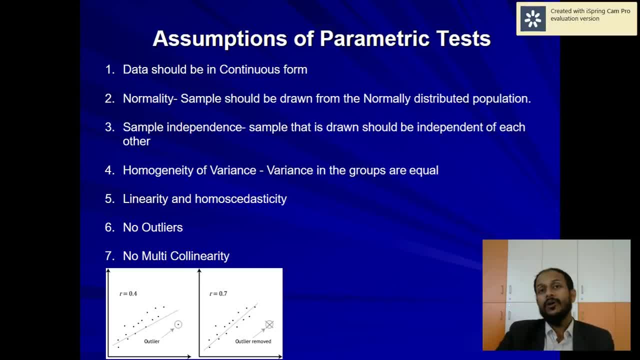 is almost touching the nearby dots. that is what we call it as linearity. if this dot, if the line, what I am drawing is in the straight line, okay. now when it comes to the homoscedasticity, when it talks about the variance, Is that variance is same across the line? okay, this is what we call it as homoscedasticity. 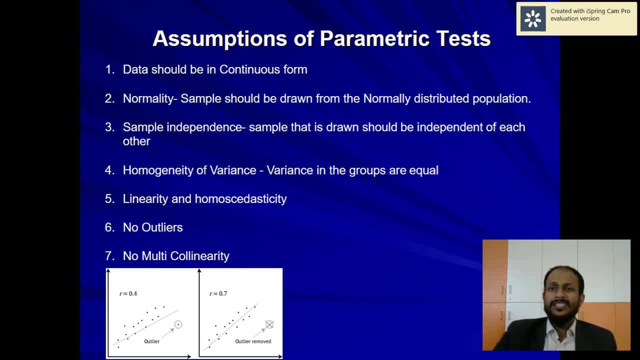 that means the dots. what I have drawn is the dots. is it almost having the same distance from the line? this is what we call it as homoscedasticity, so it should be like a tubular structure. okay, now when it comes to the outliers. now, outlier is another concept which comes under 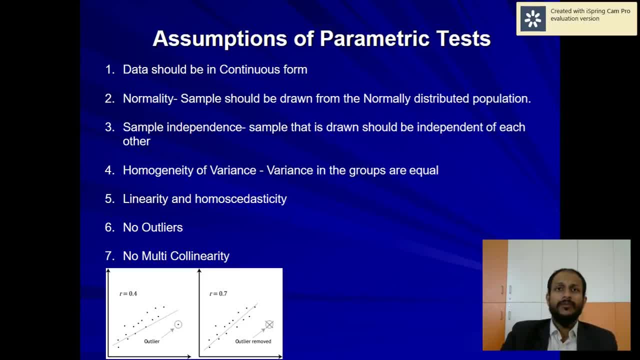 the sixth assumption of parametric test, which is also equally important. say, for example, if I am interested in calculating the Average income of Mumbai, for me Mukesh Ambani would be the outlier. so it depends upon what kind of test that you are performing and what is the objective of your research. but usually 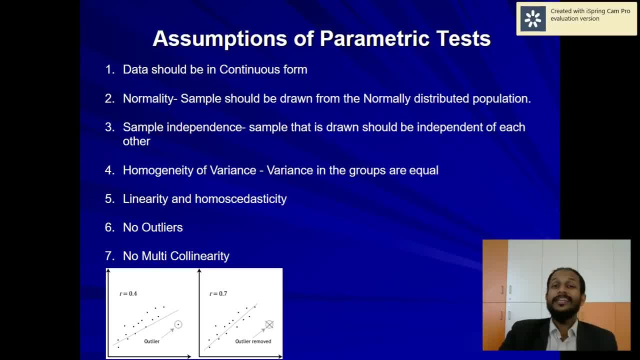 of this type of assumption usually use a test like levinis test. so whenever the p value is, we have some kind of critical and a cutoff point beyond which we fulfill the assumption of this type of test under which we reject it right. and the fourth type of assumption is all about the sorry. fifth one is: 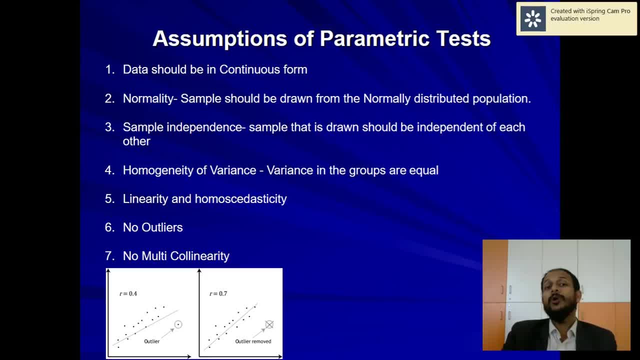 all about linearity and homoscedasticity. so now this homoscedasticity and homogeneity of variance is almost of same type. we use the word homogeneity of variance when it comes to anova and student t test, and we use the term homoscedasticity when it comes to the regression part. linearity is all. 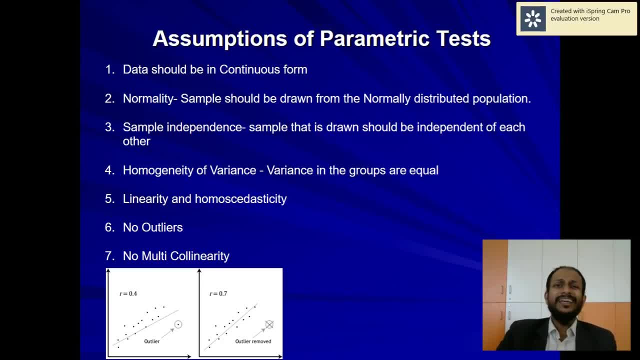 about how the variables are linearly related, if at all. i say about height and weight are related with each other. the linearity is all about to what extent that height is related with the weight in terms of linear form. if you can see the slide, you can see that the dots are present. if i am able to plot the dots, which is 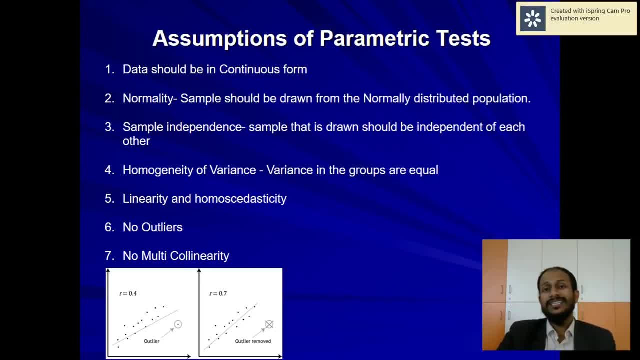 almost touching the nearby dots. that is what we call it as linearity. if this dot, if the line, what i am drawing is in the straight line, okay. now when it comes to the homoscedasticity, when it talks about the variance, is that variance is same across the line? okay, this is what we call it as homoscedasticity. 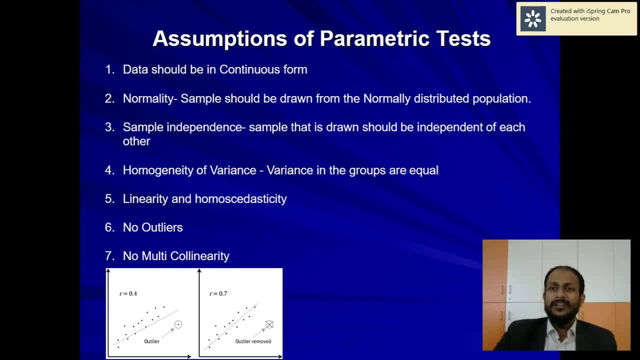 that means the dots. what i have drawn is the dots. is it almost having the same distance from the line? this is what we call it as a homoscedasticity, so it should be like a tubular structure. okay, now when it comes to the outliers. now, outlier is another concept which comes under the sixth assumption of 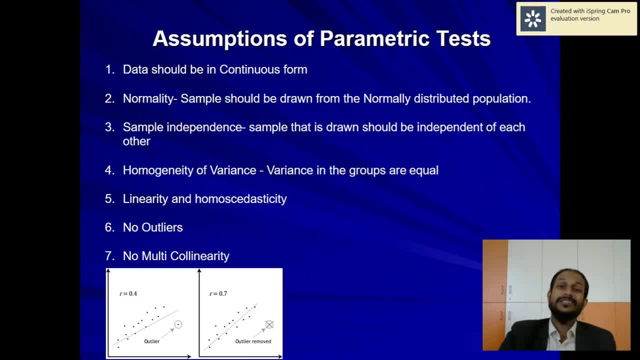 parametric test, which is also equally important. say, for example, if i am interested in calculating the average income of mumbai, for me mukesh ambani would be the outlier. so it depends upon what kind of test that you are performing and what is the objective of your research. but 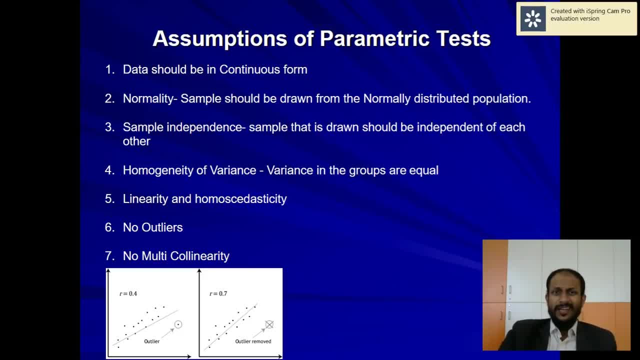 usually we try to remove the outliers. you can see that in the slide that. where do you find this kind of outliers? usually outlier we we categorize a particular variable as outlier the moment that particular variable is 3.39 standard deviation from the mean. right, sorry, 3.29 standard deviation from the mean. so we use this number as a. 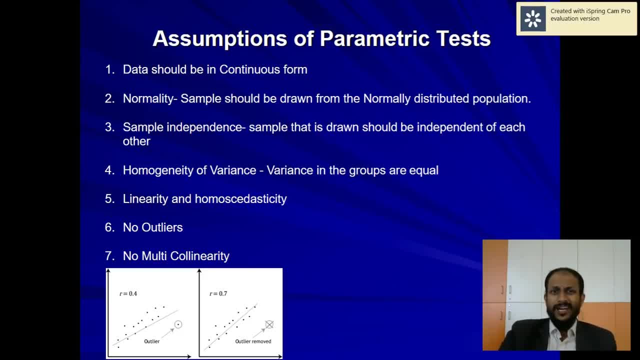 we try to remove the outliers. you can see that in the slide that. where do you find this kind of outliers? usually outlier. we categorize a particular variable as outlier the moment that particular variable is 3.39 standard deviation for the outlier. Okay, From the mean, right, so sorry, 3.29 standard deviation from the mean, so we use this number. 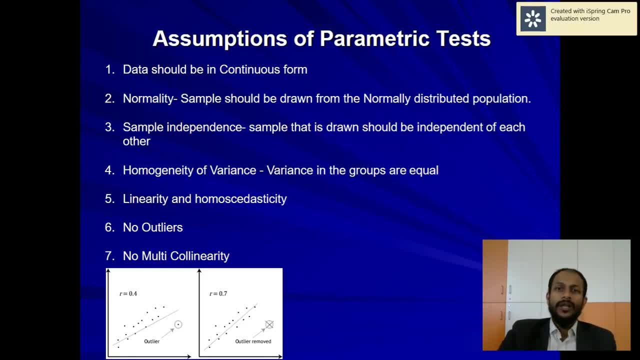 as a thumb rule so that we can categorize a particular variable as an outlier, and why it is a problem because, if at all, if you are having an outlier most of the time, we will not get a normal data and the skewness or kurtosis might not fall into the particular 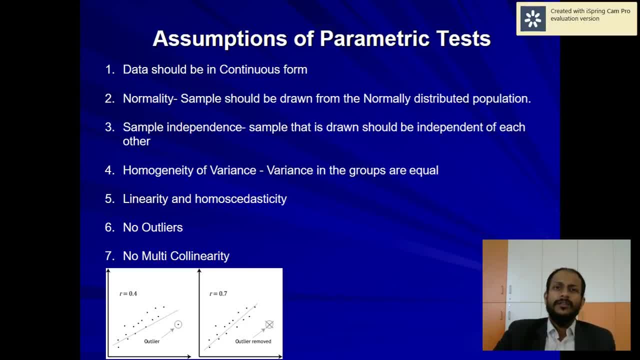 range. so sometimes we tend to take out the outlier so that we can have a normal curve, so that we can use some kind of parametric test. And the last one is: it should not have multicollinearity. what does multicollinearity? the variables should. 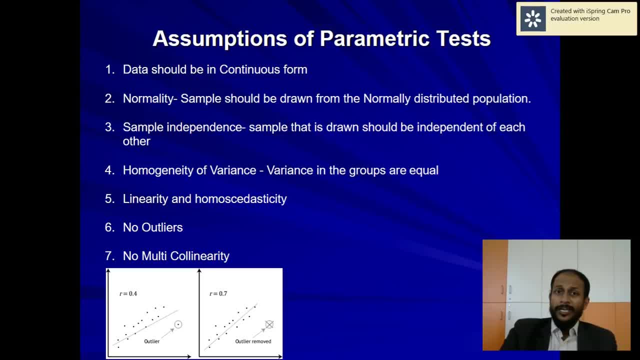 be correlated with each other. that means the independent variable should be correlated with each other, but it should not have a very high correlation. so very high correlation is always dangerous and we used, when it comes to the test, like even Cronbach, alpha when above 0.7 is good, but if it is going above 0.95 then there is doubt that it is correct. 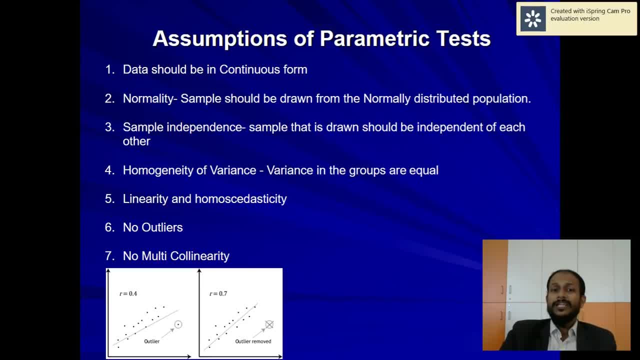 Okay, Okay, Okay- It may be doubtful, that is my data- is having multicollinearity problem, especially, we use very do importance to this concept of multicollinearity when we are using technique like regression. So before we categorize whether I am going to use parametric test or nonparametric test, 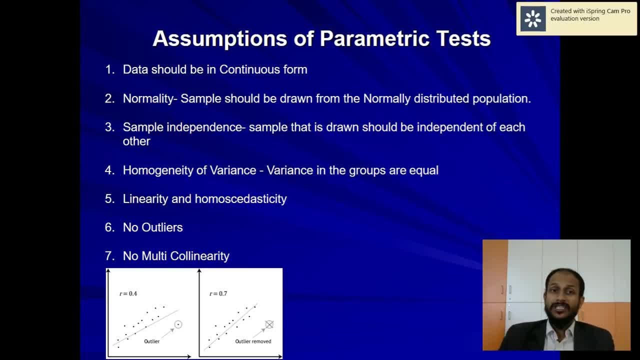 I need to perform all these seven assumptions, which is related with normality, homogeneity of variance, linearity, outlier and multicollinearity. Okay, And then I'll decide whether I'm going to use parametric test and non-parametric test. Now, in the upcoming slides, let us discuss about the different type of parametric test. 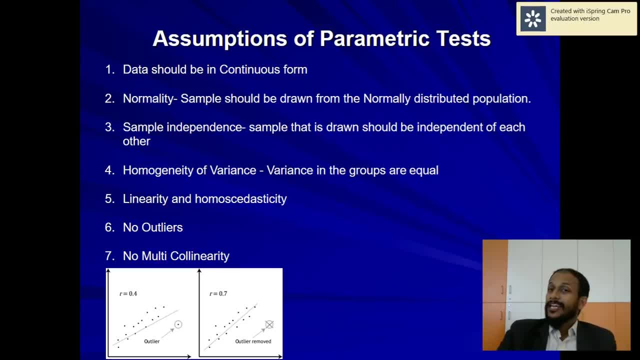 and its equivalent non-parametric test that I can use for my statistical applications, right? So the next slide is fully going to be on the part of application and what type of parametric and its equivalent non-parametric test that I can use it for my analysis, right? 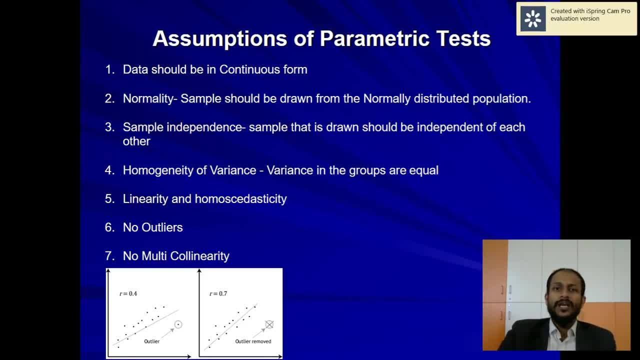 thumb rule so that we can categorize a particular variable as an outlier, and why it is a problem? because, if at all, if you are having an outlier, most of the time we will not get a normal data and the skewners or cortoses might not fall into the particular range. so sometimes we tend to take 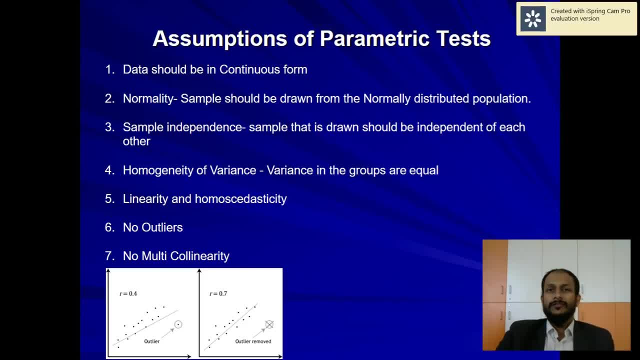 out the outlier so that we can have a normal curve, so that we can use the outlier, so that we can have a normal curve, so that we can have a normal curve, so that we can use, use some kind of parametric test. and the last one is: it should not have multicollinearity. what does? 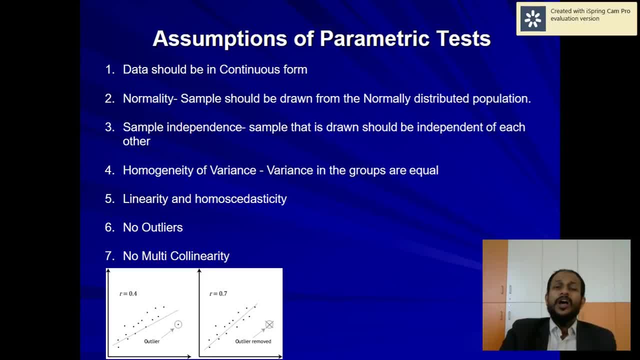 mean by multicollinearity. the variables should be correlated with each other. that means the independent variable should be correlated with each other, but it should not have a very high correlation. so very high correlation is always dangerous and we used, when it comes to the test, like even cronbach, alpha: when above 0.7 is good, but if it is going above 0.95, then there is 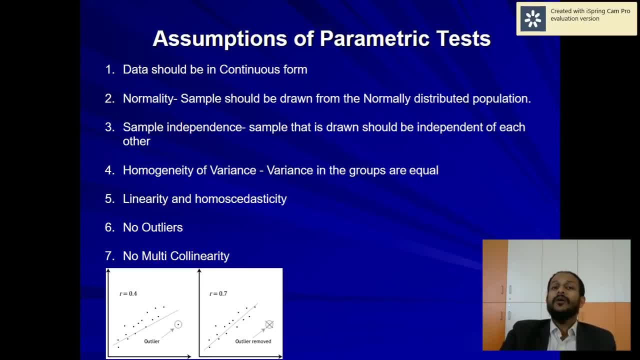 doubtful, that is, my data- is having a multicollinearity problem. especially, we use very due importance to this concept of multicollinearity when we are using technique like regression. so before we categorize whether i'm going to use parametric test or more non-parametric test, 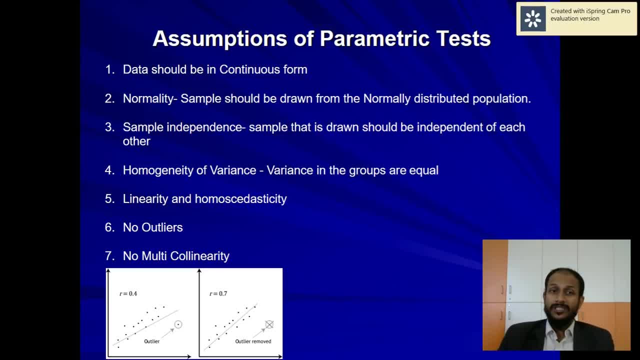 i need to perform all these seven assumptions, which is related with normality, homogeneity of variance, linearity, outlier and you multicollinearity, and then i'll decide whether i'm going to use parametric test and non-parametric test. now, in the upcoming slides, let us discuss about the different type of parametric test. 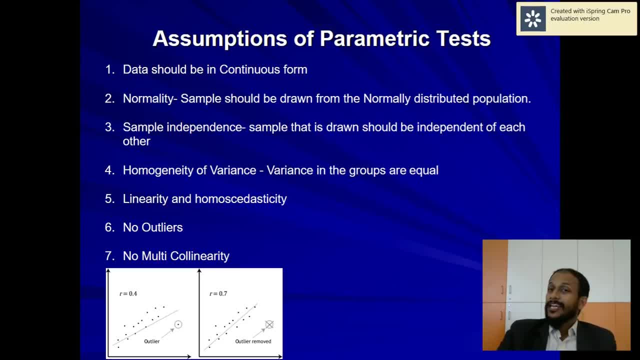 and its equivalent non-parametric test that i can use for my statistical applications. right, so the next slide is fully going to be on the part of application and what type of parametric and its equivalent non-parametric test that i can use it for my statistical applications. 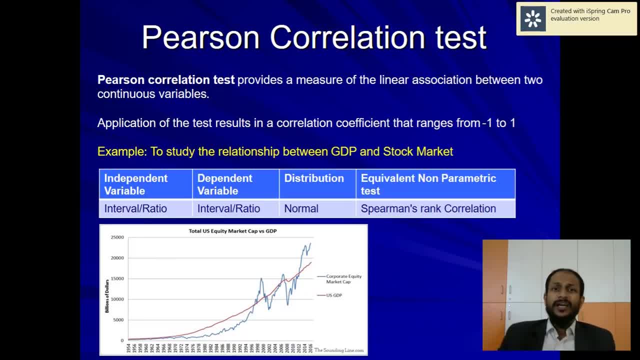 for my analysis. right, the first technique, what i'm going to discuss today, is that pearson correlation technique. now, what is pearson correlation technique? it measures the linearity between two continuous variable. say, for example, if i have two continuous variable like height and weight, so i can use pearson correlation test because both the variables are in continuous form. that 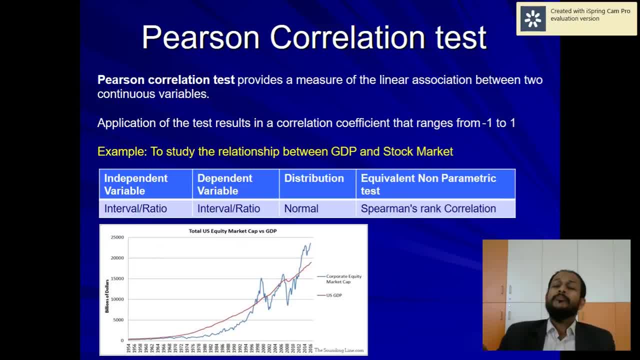 The first technique. what I'm going to discuss today is that Pearson correlation technique. Now, what is Pearson correlation technique? It measures the linearity between two continuous variable. Say, for example, if I have two continuous variable like height and weight, So I can use Pearson correlation test because both the variables are in. 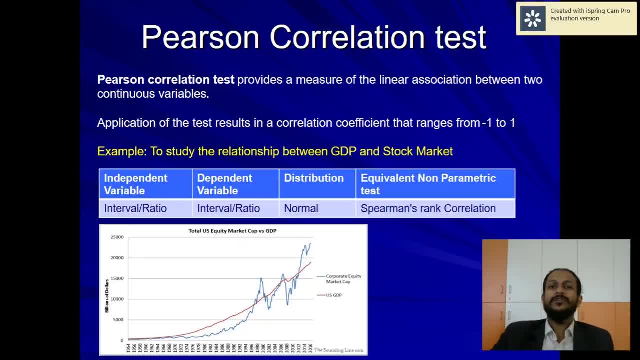 two continuous variables. Continuous form: that means it is in the ratio form, So I can use this Pearson correlation test. In this slide I have taken the example of. I wanted to study the relationship between GDP and stock market. Of course, in the shock trend- GDP and stock market- it may not have a positive correlation. 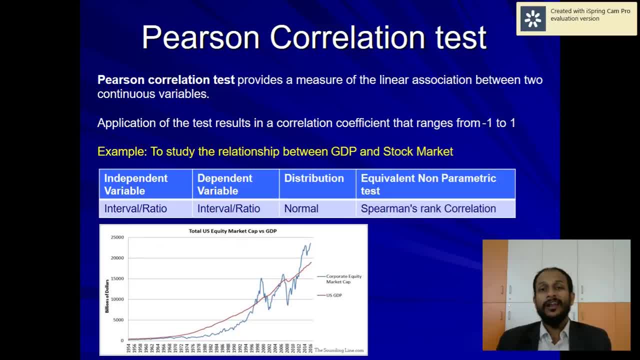 But in the long run, if you take for decades, if you take 100 year old data, you can always see that the stock market is the reflection of country's GDP. So I can say that stock market and the country's GDP is positively related with each other. 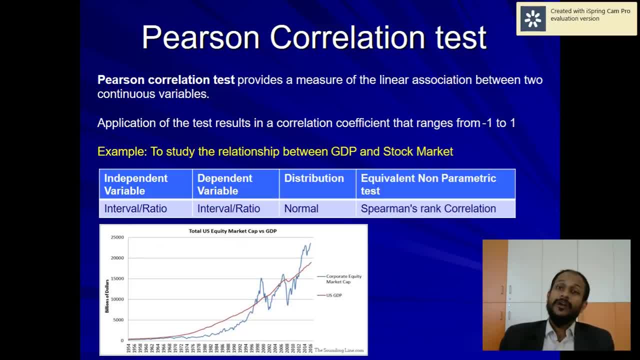 Now, when it comes to the correlation, I have a value ranging from minus one to plus one. If I'm getting a value of minus one, it indicate that it is highly negatively correlated. Plus one indicate that it is positively correlated. Zero indicate that there is no correlation between both the variables. 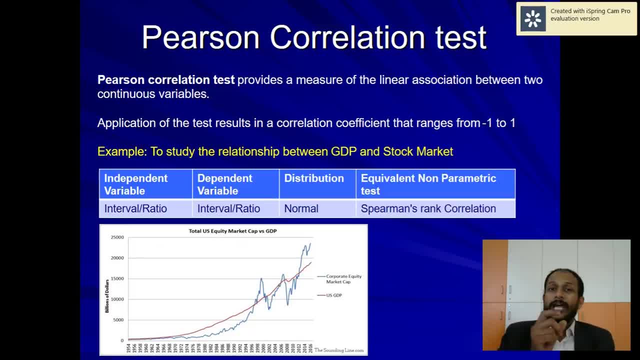 Now I have also mentioned what should be the type of correlation between the two variables, So the type of data that should be for independent variable, dependent variable and should the data should be normal or not, and its equivalent non-parametric test. that is available in front of you in the slides. 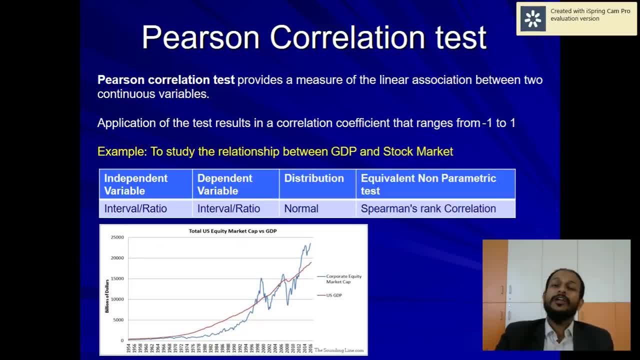 So make it simple the independent and dependent variable. it should be continuous, meaning it should be either interval or ratio. that's it. The second one is that the data should be normal. that means most of the data should be collected in the mean. 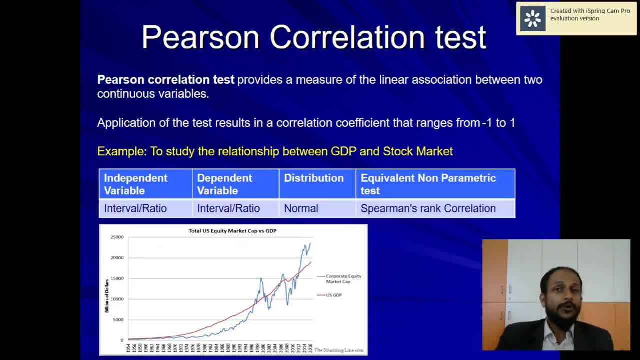 Very few data should be collected in the mean. The third one is that the data can fall on either sides. How do I check it out? Already have told you I can use tests like Shapiro-Wilcox test. I can also check it out with skewness and kurtosis. 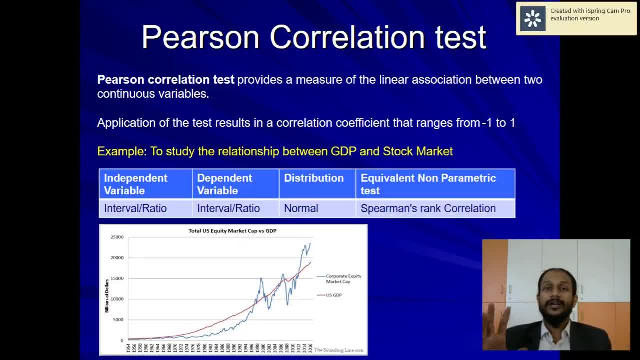 If the value is coming near to zero, then I can come to a logical conclusion that, yes, my data is approximately normal. So when these two important conditions are met, then I can also check out other conditions. Thereby I can get the confidence that, yes, I can use Pearson correlation. 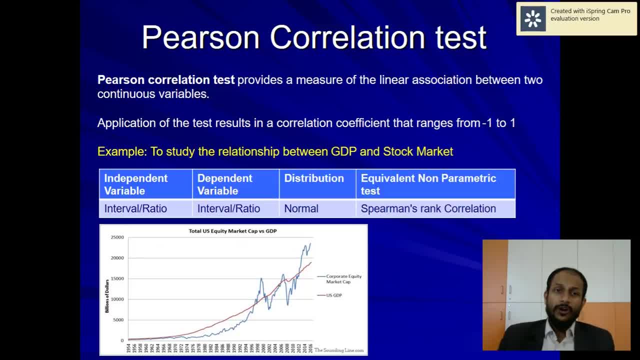 means it is in the ratio form. so i can use this pearson correlation test. in this slide i have taken the example of. i wanted to study the relationship between gdp and stock market. of course, in the shock trend- gdp and stock market- it may not have a positive correlation. but in the long run, if you take for decades, if you take 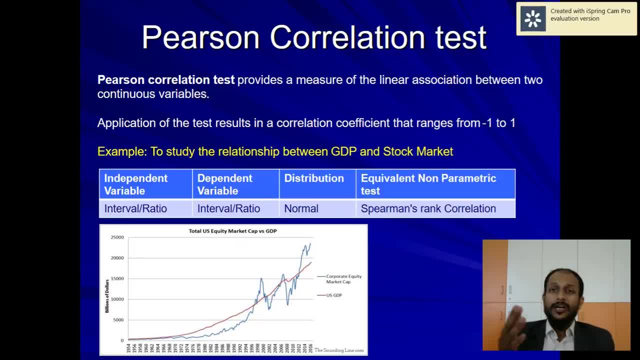 100 year old data, you can always see that the stock market is the reflection of country's gdp, so i can say that stock market and the country's gdp is positively related with each other. now, when it comes to the correlation, i have a value ranging. 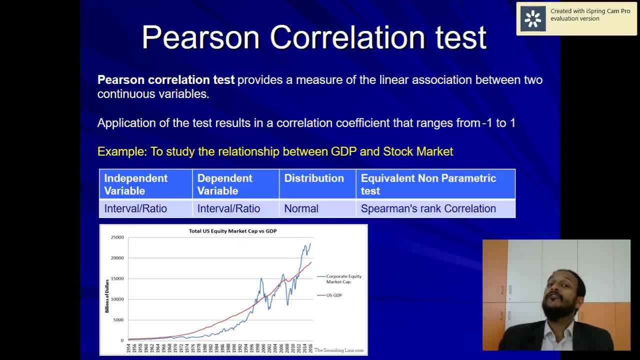 from minus 1 to plus 1. if i'm getting a value of minus 1, it indicate that it is highly negatively correlated. plus 1 indicate that it is positively correlated. 0 indicate that there is no correlation between both the variables. now i have also mentioned what should be the type of data that. 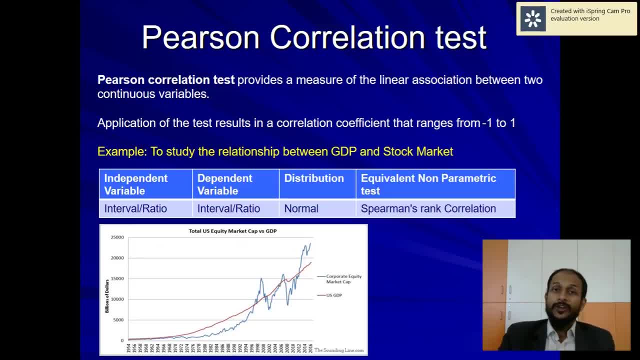 should be for independent variable and should the data should be normal or not, and its equivalent non-parametric test. that is available in front of you in the slides. so make it simple: the independent and dependent variable. it should be continuous, meaning it should be either interval or ratio. that's it. the second one is that the data 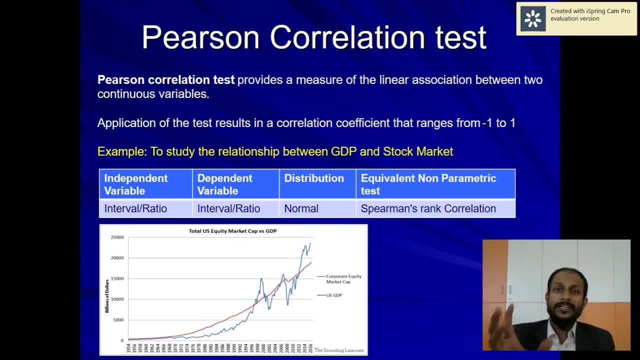 should be normal. that means most of the data should be collected in the mean. very few data can fall on either sides. how do i check it out? already i have told you i can use tests like shapiro wilcox test. i can also check it out with. 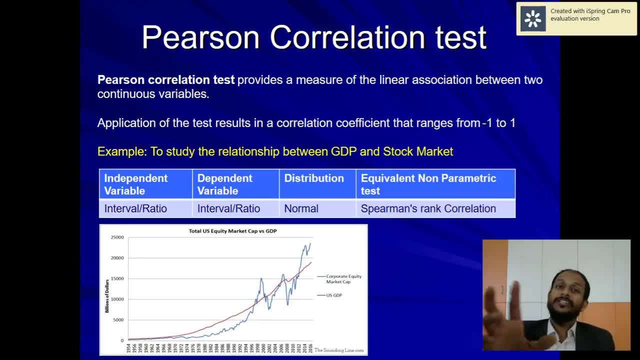 you know i mean skewness and kurtos risk. if the value is coming near to zero, then i can come to a logical conclusion that, yes, my data is approximately normal. so when these two important conditions are met, then i can also check it out other conditions thereby i can. 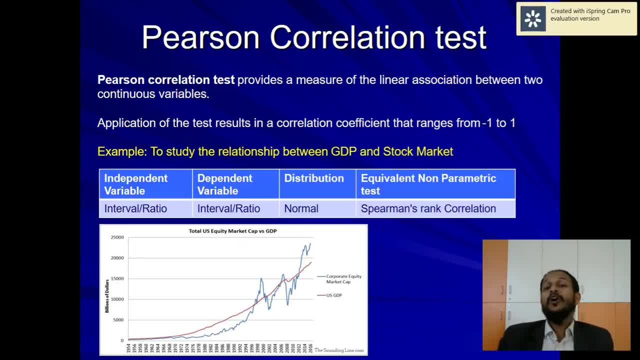 get the confidence that, yes, i can use pearson correlation test. if any one of these assumptions are getting violated, don't worry. we always have an equivalent non-parametric test called spearmint rank correlation. i'm not going to explain fully about the spearmint rank correlation, but understand that if my 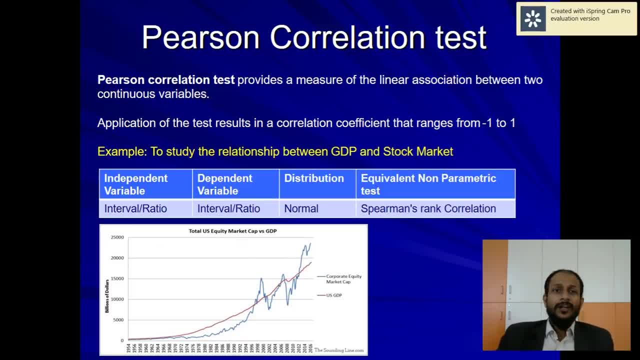 If any one of these assumptions are getting violated, don't worry. we always have an equivalent non-parametric test called Spearman-Rank correlation. I'm not going to explain fully about this Spearman-Rank correlation, but understand that if my data is not normal, what do I do? 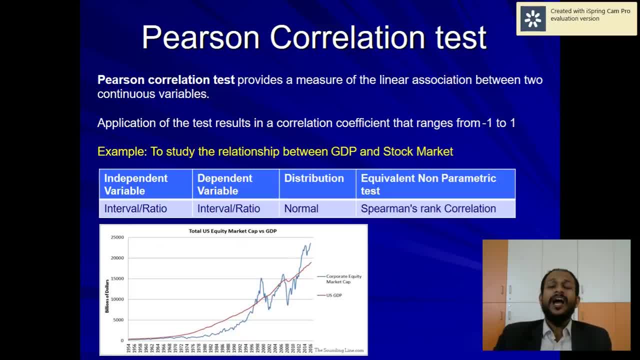 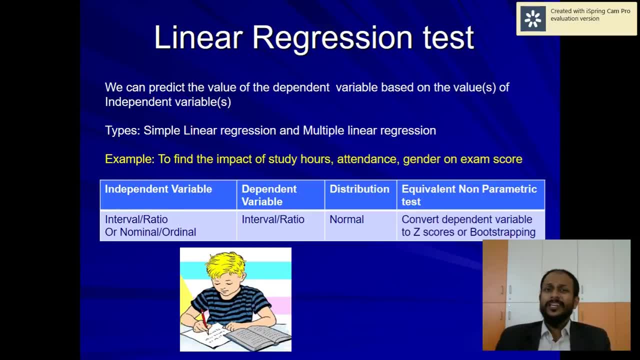 I convert the data into rank and through that rank, I use this type of Spearman-Rank correlation. OK, let's get into the second technique. Second technique: I use something called linear regression. Now, when it comes to the linear regression here, what do I do? 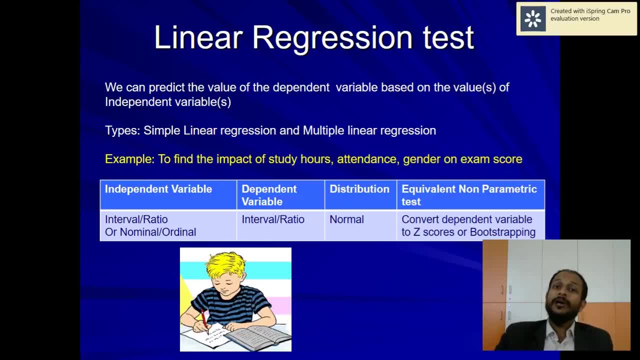 I predict the dependent variable through the available independent variable. Now linear regression test. most of the time I use it mainly for prediction purpose. Now, when it comes to linear regression, here also I do have two types of linear regression test. One is that simple linear regression. 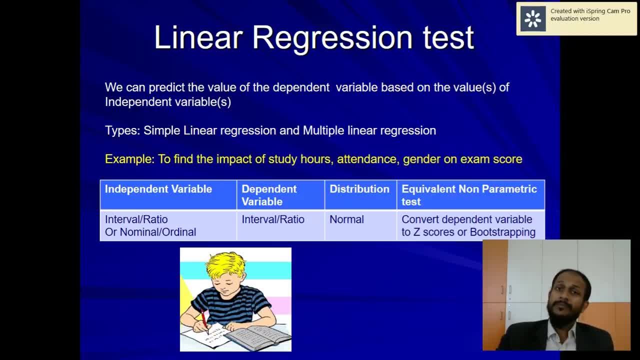 Another one is that multiple linear regression. What does mean by simple linear regression? When I'm trying to find out the impact of one independent variable on the one dependent variable, I use a technique called simple linear regression. Say, for example, I'm studying the relationship between salary and job satisfaction. 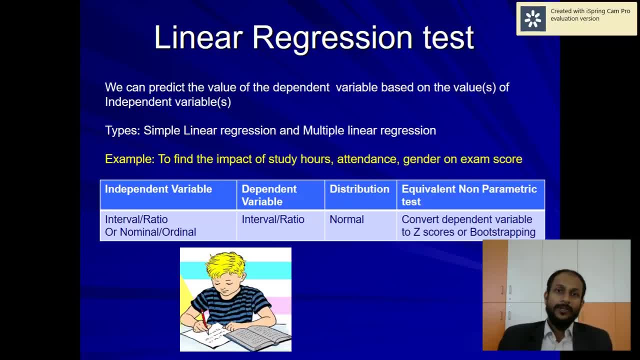 Salary could be an independent variable, Job satisfaction could be a dependent variable And I'm trying to find out the strength of the impact. That time I can use a technique called simple linear regression. What is multiple linear regression? Multiple linear regression is a technique called simple linear regression. 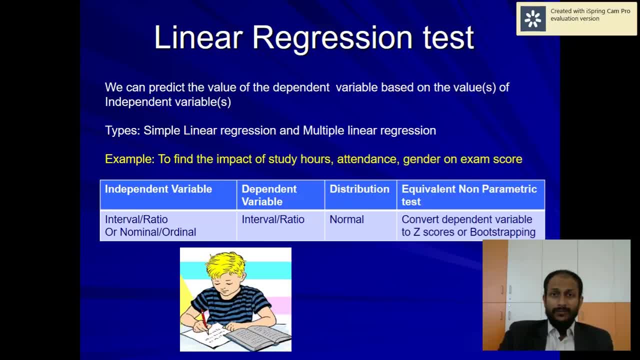 Simple linear regression is something. when I'm trying to find out the strength of the impact of multiple independent variables, two or more than two- That time I'm using a technique called multiple linear regression. OK, I have given you one example. Let's say that we wanted to study the impact of study hours and attendance and gender on examination score. 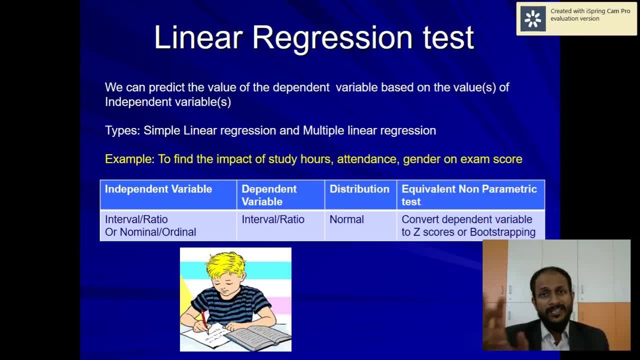 Now, here you can see that there are three independent variables: One, study hours, Second, attendance, And third is gender and its impact on examination score. Now, this, I have clearly mentioned it in the form of what should be the characteristics of independent variable, dependent variable. 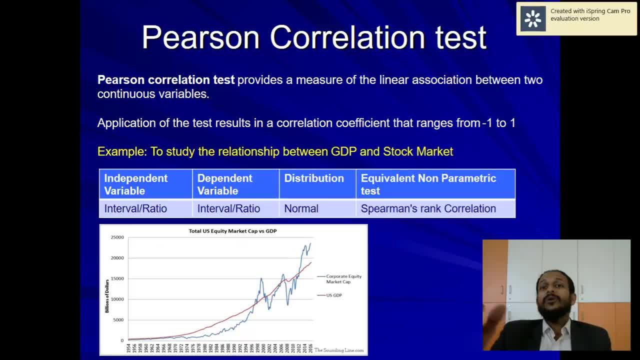 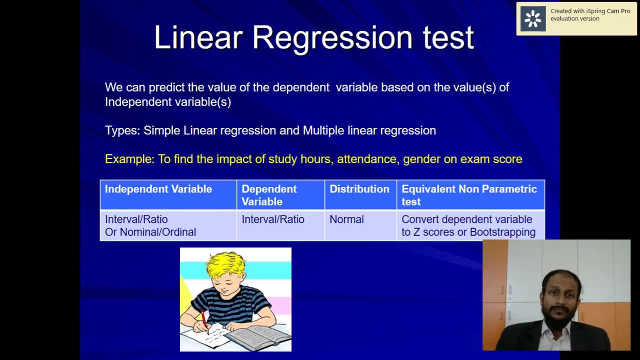 data is not normal. what do i do? i convert the data into rank and through that rank, i use this type of spearmint rank correlation. okay, let's get into the second technique. second technique: i use something called linear regression. now, when it comes to the linear regression, 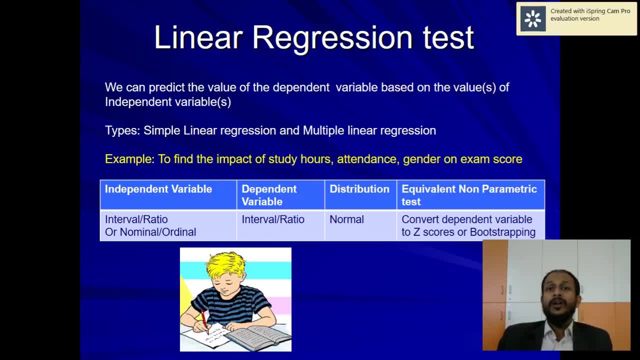 here. what do i do? i predict the dependent variable through the available independent variable. now linear regression test. most of the time i use it mainly for prediction purpose. now, when it comes to linear regression, here also i do have two type of linear regression test. one is that simple linear regression. another one is that multiple linear regression. like what? 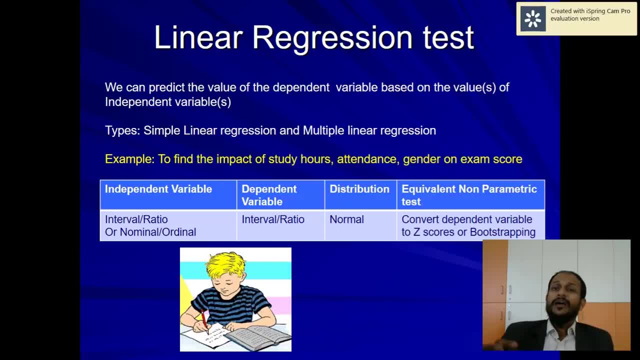 does mean by simple linear regression. when i'm trying to find out the impact of one independent variable on the one dependent variable, i use a technique called simple linear regression. say, for example, i'm studying the relationship between salary and job satisfaction. salary could be an independent variable, job satisfaction could be a dependent variable, and i'm trying 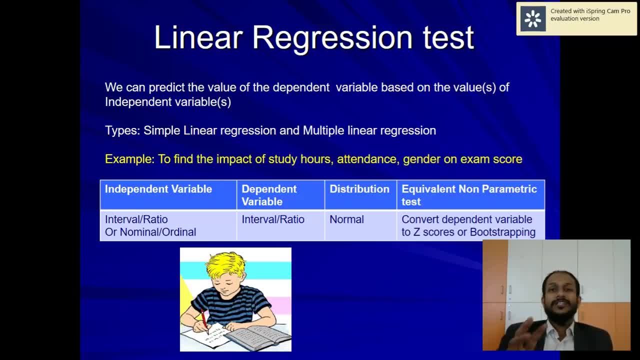 to find out the strength of the impact, that time i can use a technique called simple linear regression. what is when we multiple linear regression? multiple linear regression is something when i'm trying to find out the strength of the impact of multiple independent variables, two or more than two. that time i'll be using a technique called multiple linear. 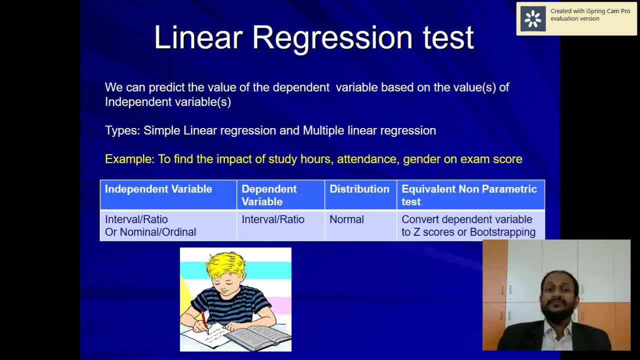 regression. okay, i have given you an example. let's say that we wanted to study the impact of study hours and attendance and gender on examination score. now here you can see that there are three independent variables: one, study hours, second, attendance, and third is gender and its impact on examination score. now, this i have clearly mentioned it in in. 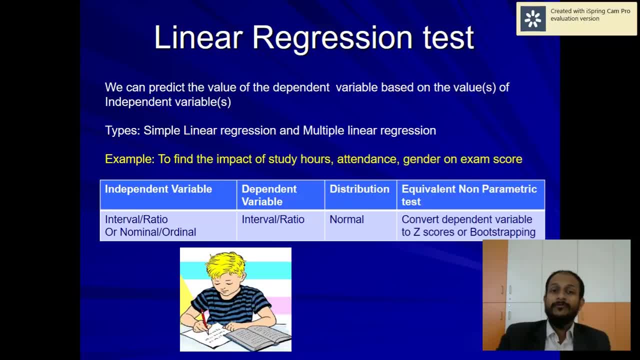 the form of what? what should be the characteristics of independent variable, dependent variable, what about the distribution and stuff like that? in this slide you can see that when it comes to the dependent variable, it should be continuous data. that means either it should be interval scale or it should be a ratio scale. and when it comes to the independent 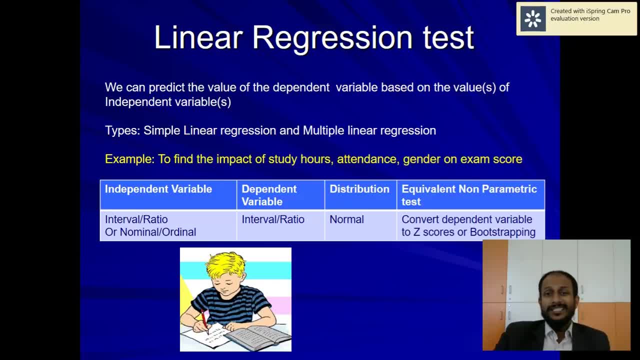 What about the distribution and stuff like that? in this slide You can see that when it comes to the dependent variable, it should be continuous data. That means either it should be interval scale or it should be a ratio scale. And when it comes to the interval scale, it should be a ratio scale. 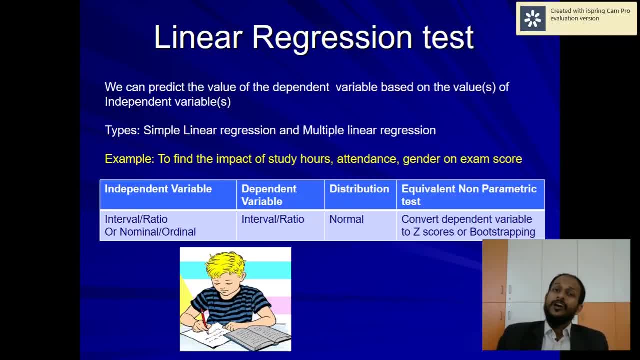 Independent variable. it can be interval scale, ratio scale or nominal or ordinal scale, not a problem, We have that flexibility. We use some technique called dummy variable technique, through which we can come to a conclusion that what is the strength of the impact that independent variable is having on dependent variable, even if the independent variable is categorical? 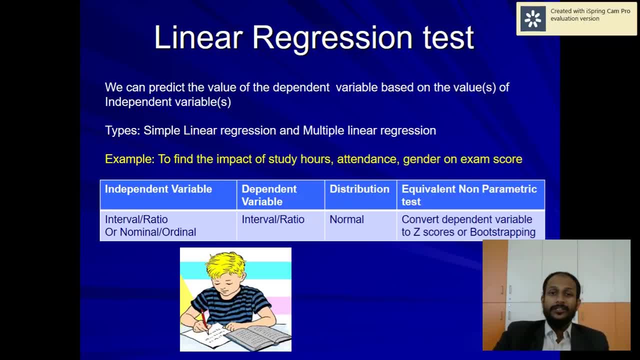 That is not at all a problem, that we can use it through this linear regression technique and the distribution. What I'm having. It should be normal. There is no compromise on it. Now, what if these assumptions are not being met? Not only these assumptions. discuss about the assumptions, seven assumptions that I have discussed in the beginning of the session. 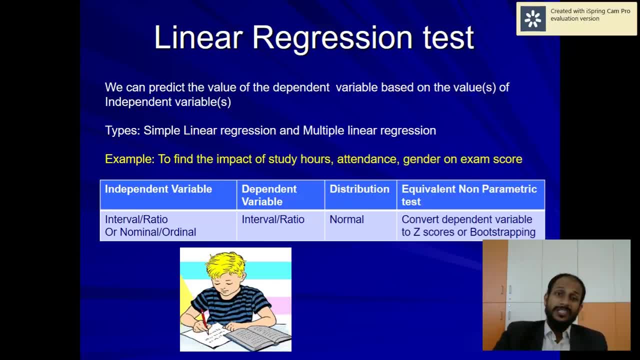 All these seven assumptions has to be met so that we can use these type of tests. What if it is not getting met? Then the best way is that you try converting your dependent variable, in case, if it is not normal, to a normal variable. How do I do that? 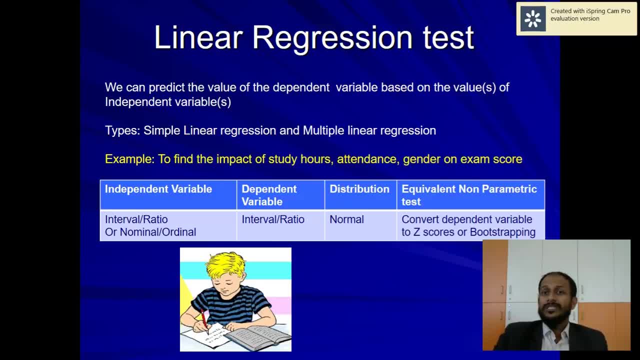 We use a few algorithms, We use some technique like Z scores, which is available in SPSS and other softwares, and through the Z score We will be able to get a normal distribution so that I can get the first assumption of this. It is a normality test and I can also take out some of the outliers and thereby I can use this linear regression test. 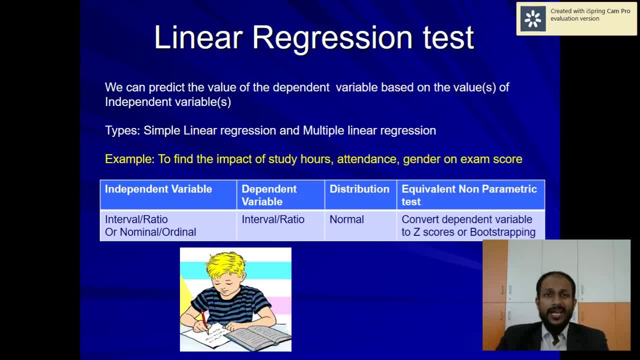 Otherwise, one of the technique which other researchers uses is that you can also use a technique called Bootstrapping. So bootstrapping is another technique which cannot be explained it in this session. that will have a separate session. We can discuss about the bootstrapping technique. 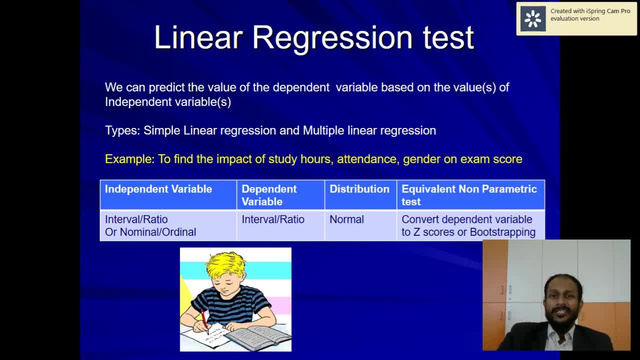 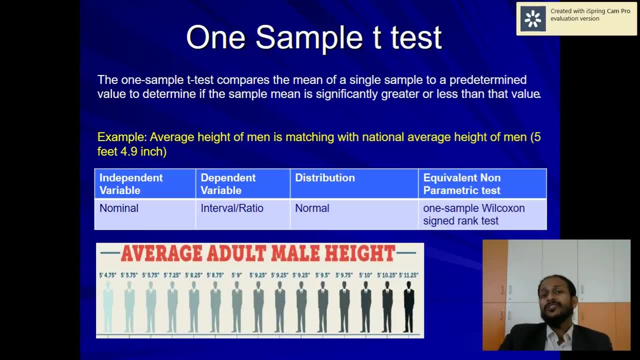 Now, this is what all about when it comes to the linear regression test. OK, the third technique which we can discuss is one sample t-test. Now, when it comes to the one sample t-test, it compares the means of a single sample to a predetermined value to determine. 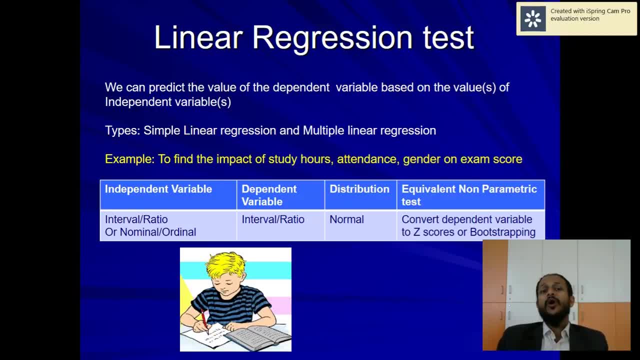 variable. it can be interval scale, ratio scale or nominal or ordinal scale, not a problem, we have that flexibility. we use some technique called dummy variable technique, through which we can come to a conclusion that what is the strength of the impact that independent variable is having a depend on dependent variable, even if the independent variable is categorical? 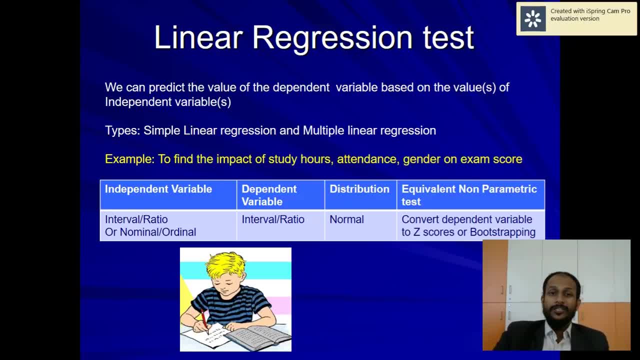 that is not at all a problem, that we can use it through this linear regression technique and the distribution. what i'm having. it should be normal. there is no compromise on it. now, what if these assumptions are not being met? not only these assumptions discuss about the assumption. seven assumptions that i have discussed in 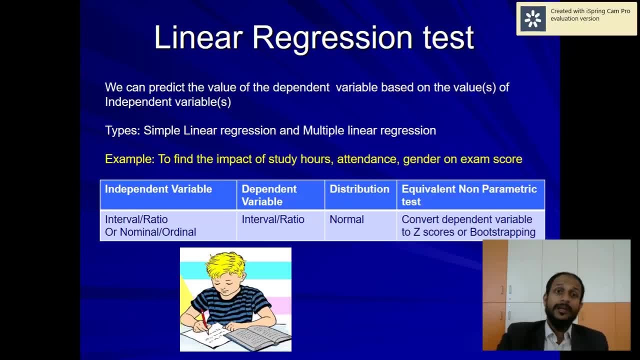 the beginning of the session. all these seven assumptions has to be met so that we can use these type of tests. what if it is not getting met? then the best way is that you try converting your dependent variable, in case, if it is not normal, to a normal variable. how do i do that? 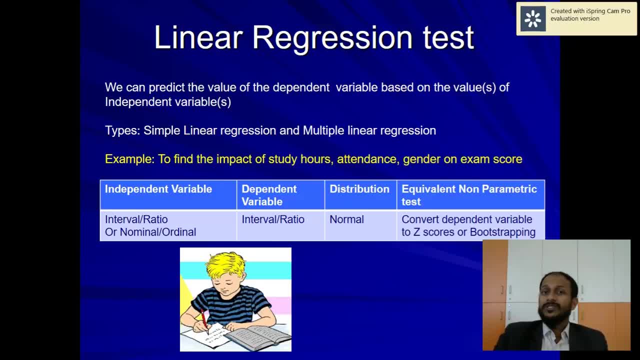 we use a few algorithms, we use some technique like z-scores, which is available in spss and other softwares, and through that z-score we will be able to get a normal distribution so that i can get the first assumption of yes, it is a normality test, and i can also take out some 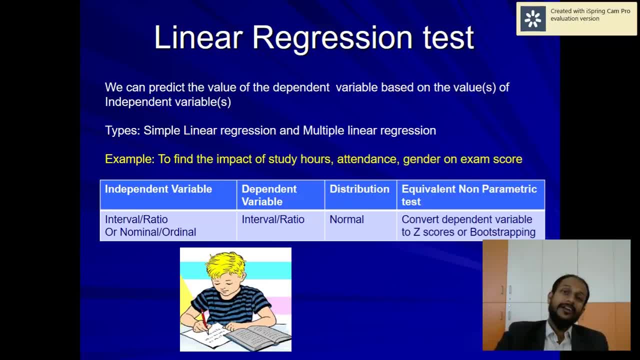 of the outliers and thereby i can use this linear regression test. otherwise, one of the technique which other researcher uses is that you can also use a technique called bootstrapping. so do. bootstrapping is another technique which cannot be explained it in this session. that will have a separate. 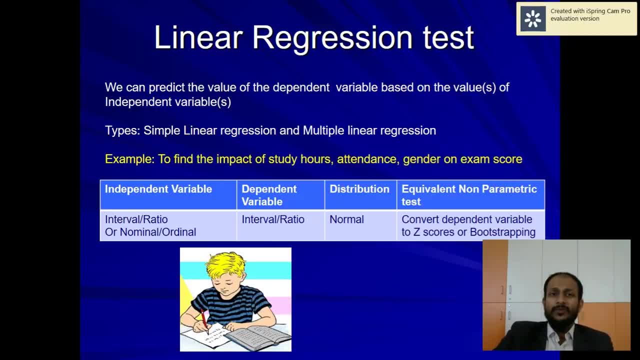 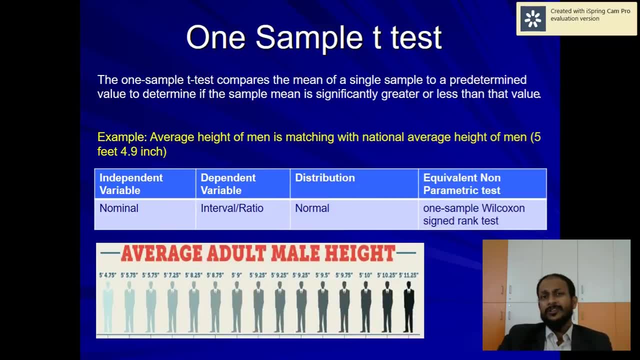 session. we can discuss about the bootstrapping technique. now, this is what all about when it comes to the linear regression test. okay, the third technique which we can discuss is one sample t-test. now, when it comes to the one sample t-test, it compares the means of. 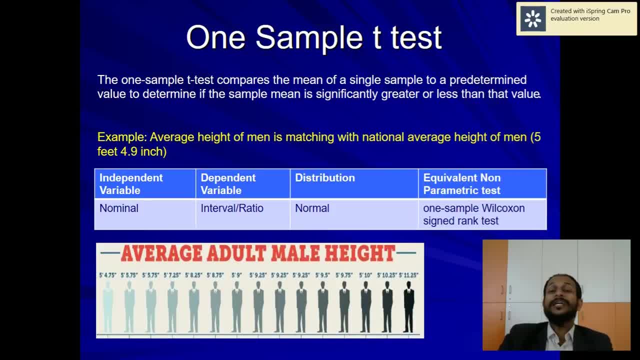 a single sample to a pre-determined value to determine if the sample mean is significantly greater than or lesser than the particular value. say, for example, i have some hundred men and i wanted to check whether the average height of all the hundred men is equivalent to the national average. 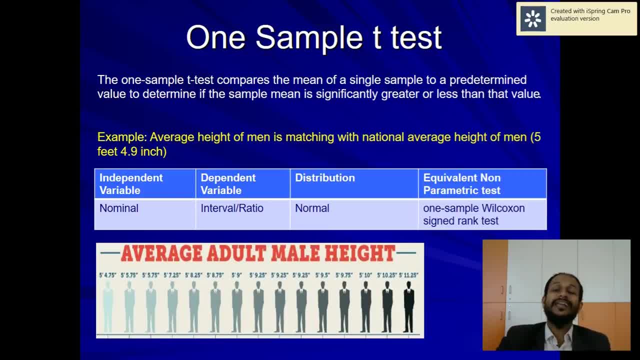 If the sample Mean is significantly greater than or lesser than the particular value Say. for example, I have some hundred men and I wanted to check whether the average height of all the hundred men is equivalent to the national average. The national average of men is five feet and four point nine inch. 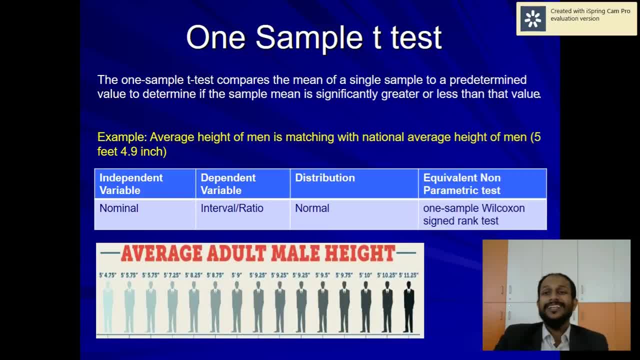 Let's say that I have calculated. the average height of this man is five feet and three inches. Now I wanted to check Whether is this matching with the national average of men. Now, if at all, if this is my application, the kind of test that I can use for this application is one sample t-test. 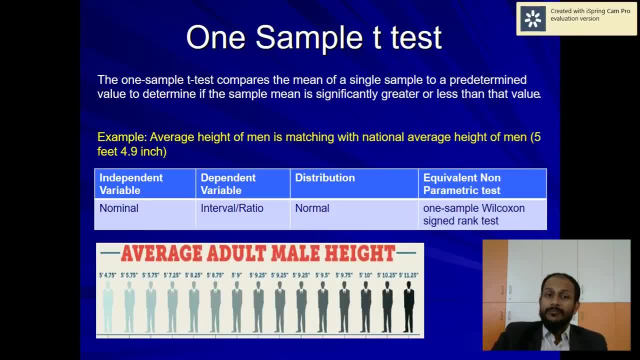 I have also mentioned what should be the scale of independent variable. What should be the scale of dependent variable? OK, in this particular set of course. Yes, the dependent variable should be continuous. That means it should be either interval or ratio. 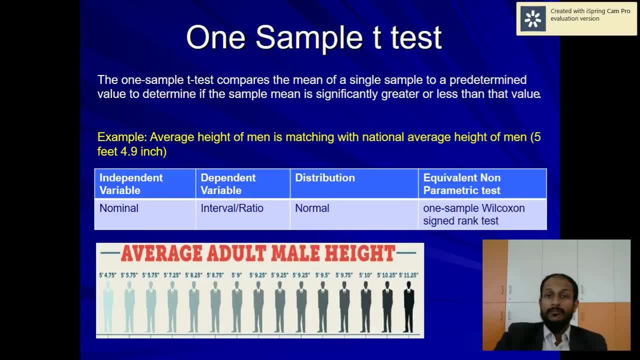 And the dependent variable should be normal data of the dependent variable. Of course it should be normal data and it should also fulfill all the other assumptions of parametric test. then I can use one sample t-test. If not, if I am not able to meet the other assumptions of parametric test, 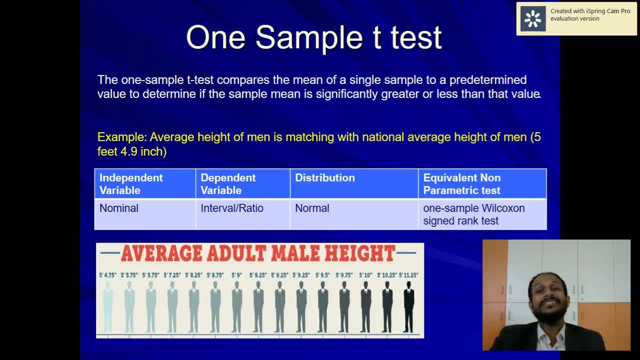 I have an equivalent test called one sample, Wilcoxon signed rank test. Now this alternate technique I can use, so don't get disheartened If your data is not able to fulfill the assumptions of parametric test. one way is that you can convert your data to a normal data by using z-score. 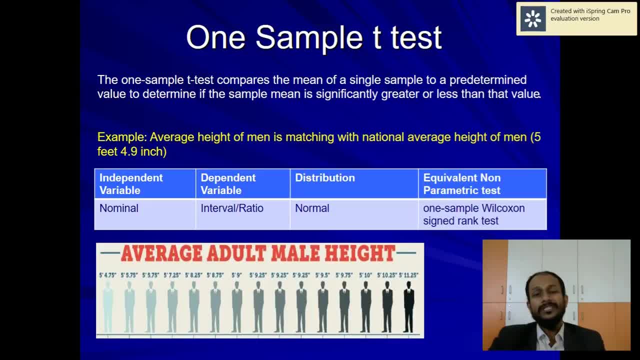 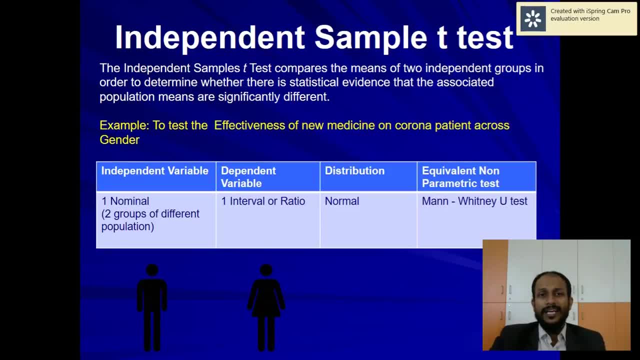 Another way is that, instead of using parametric test, you can use its equivalent non-parametric test. So the choice is yours. Now let us get into another technique. The other test is independent sample t-test. Now, this independent sample t-test: it compares the means of two. 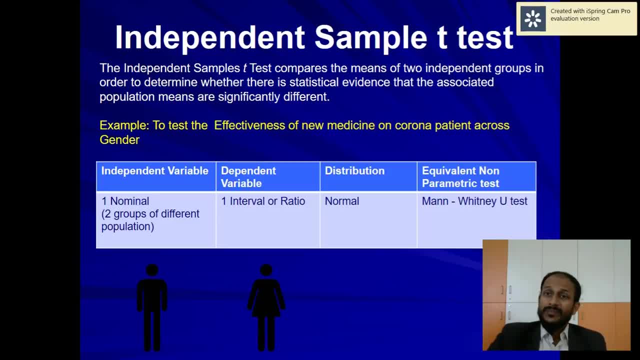 independent group to determine which mean is significantly different from the other means. To make it very simple, it compares the means across two different groups of population. I have used the word two different means of two different populations, So I am not talking about the same population. 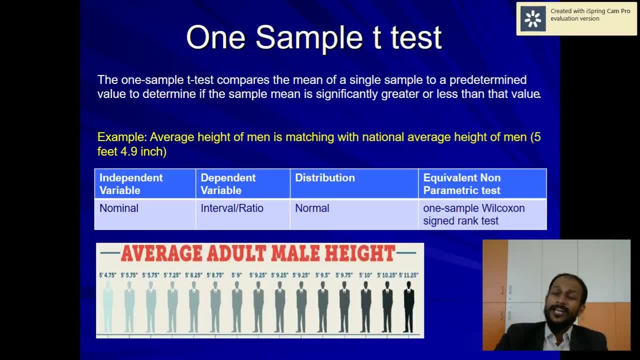 the national average of men is 5 feet and 4.9 inch. let's say that i have calculated. the average height of this man is 5 feet and 3 inches. now i wanted to check whether is this matching with the national average, and i have calculated. the average height of this man is 5 feet and 3 inches. 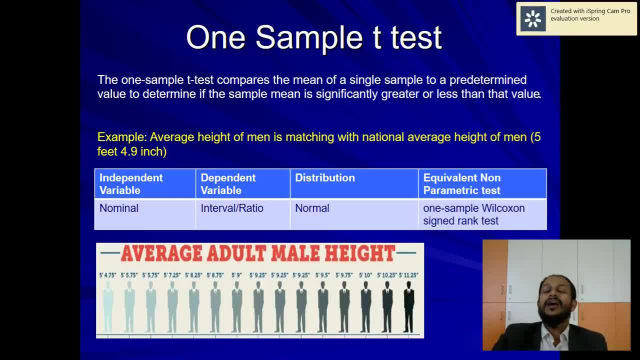 now, if at all, if this is my application, the kind of test that i can use for this application is one sample t-test. i have also mentioned what should be the scale of independent variable. what should be the scale of dependent variable. okay, in this particular site, of course, yes, the 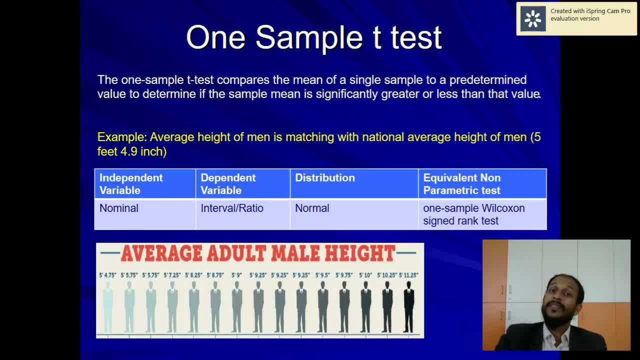 dependent variable should be continuous. that means it should be either interval or ratio and the independent variable should be normal data of the dependent variable. of course it should be normal data and it should also fulfill all the other assumptions of parametric test. then i can use one sample t-test. if not, if i am not able to, 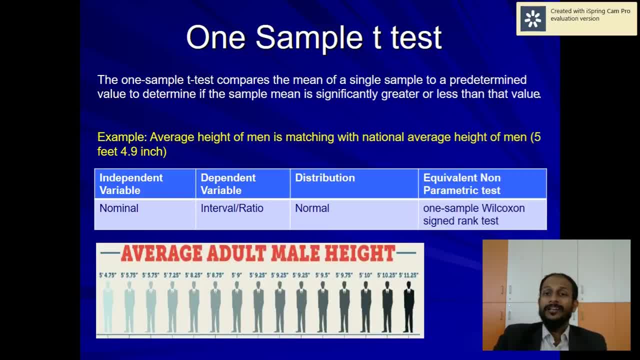 meet the other assumptions of parametric test. i have an equivalent test called one sample wilcoxon signed rank test. now this alternate technique i can use, so don't don't get disheartened if your data is not able to fulfill the assumptions of parametric test. so i can use one sample t-test. 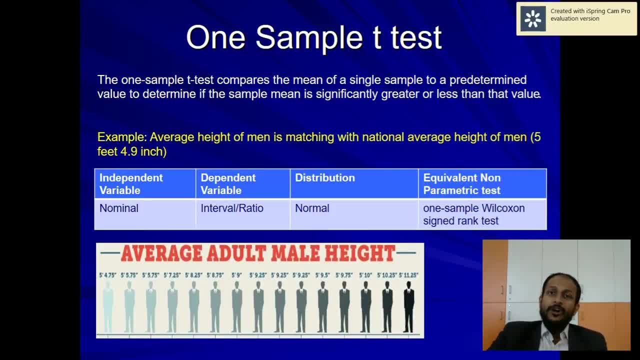 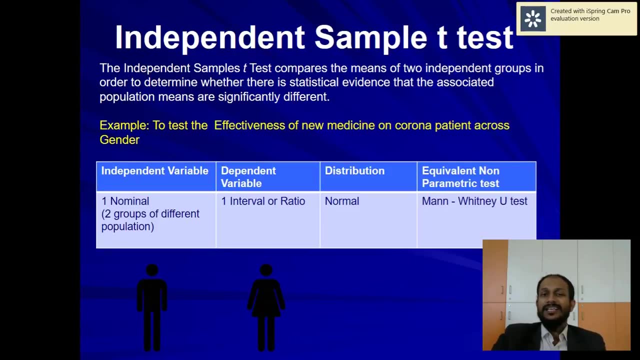 one way is that you can convert your data to a normal data by using z-score. another way is that, instead of you using parametric test, you can use its equivalent non-parametric test. so the choice is yours. now let us get into another technique. the other test is independent sample t-test. now, 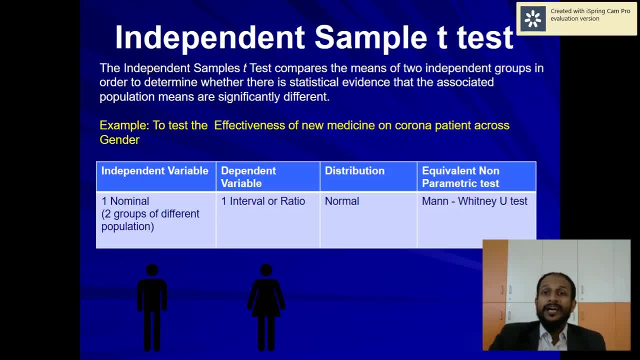 this independent sample t-test. it compares the means of two independent group to determine which which mean is significantly different from the other mean. to make it very simple, it compares the means across two different groups of population. right, i have used the word two different means of two different populations, so i am not talking about the same population. it should. 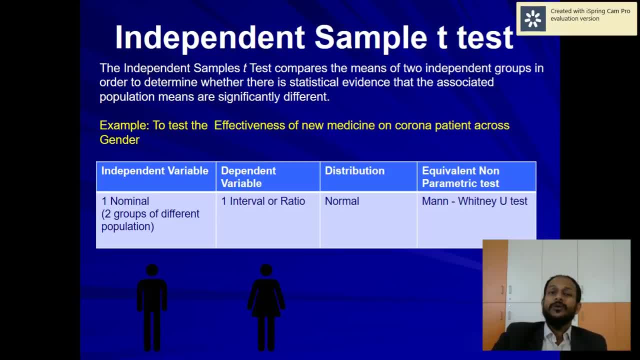 be different population. let me give you an example so that you can have a better understanding on this topic. say, for example, i have a new medicine for corona and i wanted to check is this medicine is effective among people. so now for that, what do i do? i take two. i take gender as a criteria. 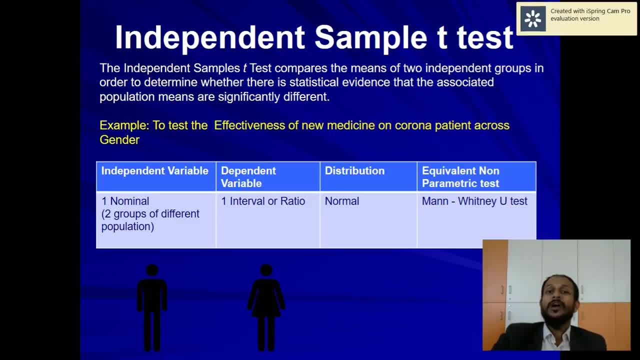 It should be different population. Let me give you an example so that you can have a better understanding on this topic. Say, for example, I have a new medicine for Corona and I wanted to check if this medicine is effective among people. So now, what do I do? 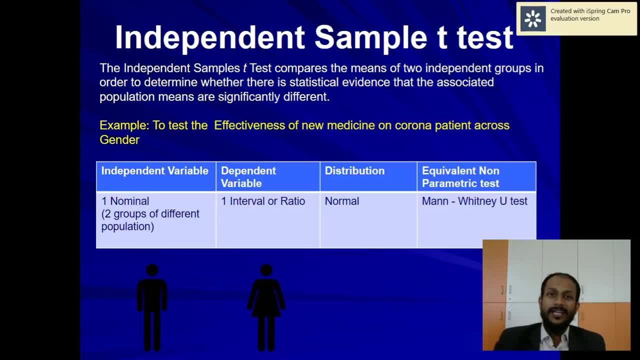 I take two. I take gender as a criteria and I give the medicine to 100 males and 100 females and I'm checking how is the recovery rate among the men and how is the recovery rate among the women. That means I'm actually checking that who is recovering faster? 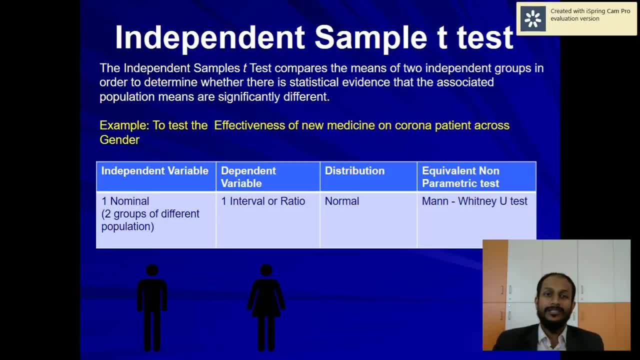 Is men is recovering faster or is it women is recovering faster? Now, how do I check it out? I check their body temperature. Now, when I'm doing these type of tests where I compare the mean of the body temperature across two different groups, 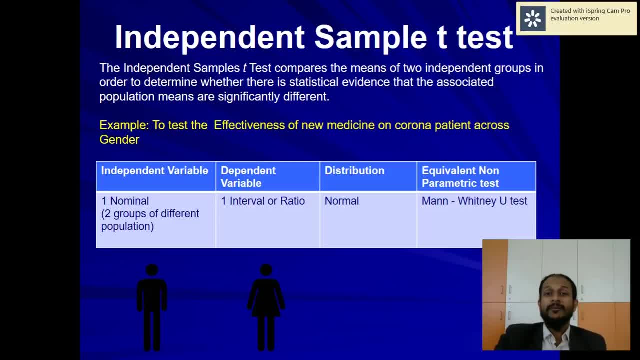 that type of test. what I'll be using is independent sample t-test. I've also given what should be the characteristics of independent variable- dependent variable- in the slide. you can refer it, And I have given it in the way that you can feed this data in SPSS. 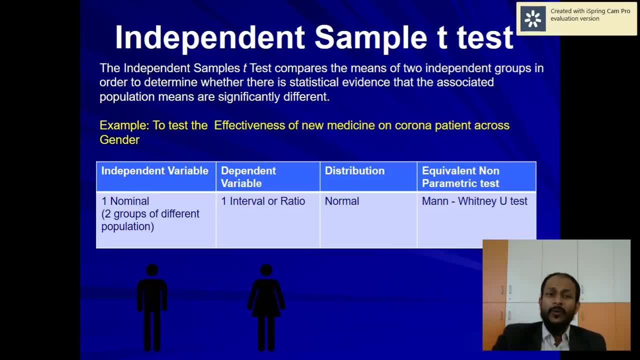 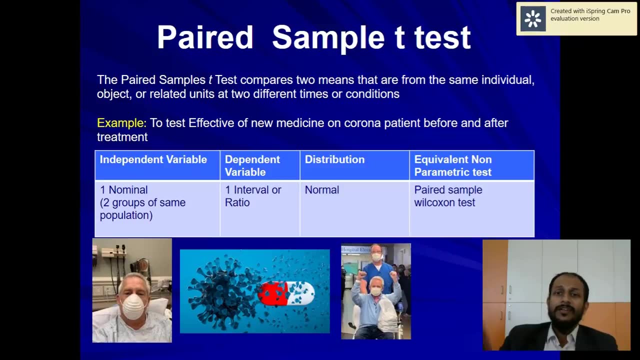 That means I have mentioned, if it does one group under one group, you have two groups of different population like this. OK, now I've also mentioned the equivalent nonparametric test, man witness u-test. OK, fine, Let us discuss about the pad sample t-test, the other technique. 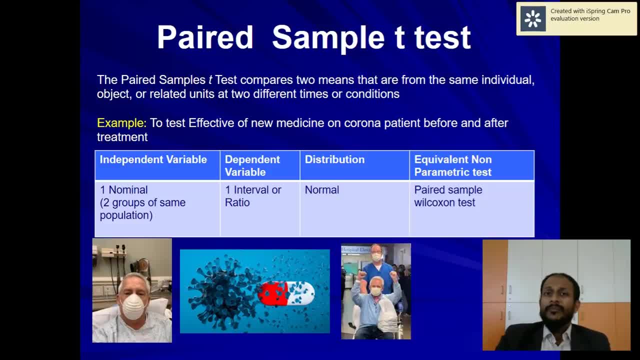 Now here in pad sample t-test we compare the means of the same population. Look at the difference between independent sample t-test and pad sample t-test. In independent sample t-test I am comparing the means across two different population. In pad sample t-test I am comparing the means across two samples of the same population. 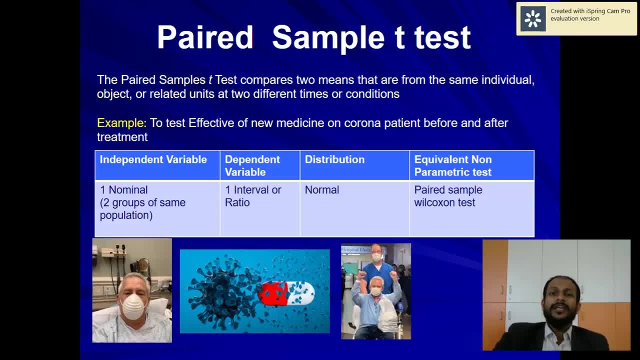 Now let me explain it. Say, for example- here also I am taking this corona as an example I wanted to have- I am checking the new medicine of corona across patient before and after the treatment. Now, most of the time I use this pad sample t-test in terms of conditions or in terms of situation. 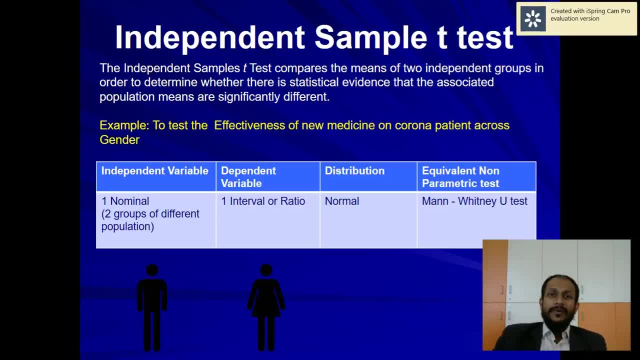 and i give the medicine to hundred males and hundred females and i'm checking how is the recovery rate among the men and how is the recovery rate among the women. that means i am actually checking that who is recovering faster. is men is recovering faster, or is it women is? 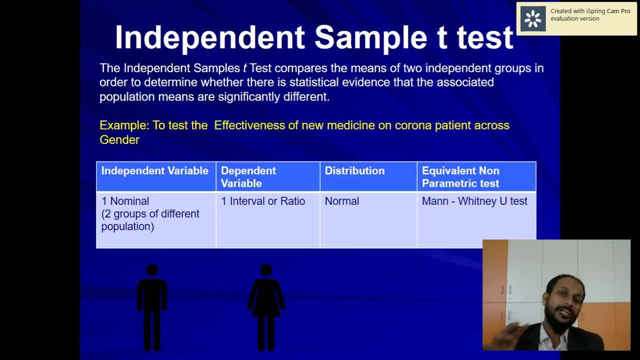 recovering faster. now how do i check it out? i check their body temperature. now, when i am doing these type of test where i compare the mean of the body temperature across two different groups, that type of test what i'll be using is independent sample t-test. i have also given what should be the characteristics of independent variable. dependent variable. 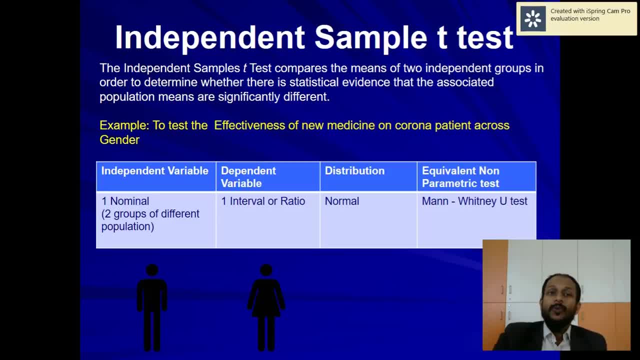 in the slide. you can refer it and i have given it in the way that you can feed this data in spss. that means i mentioned it does one group under one group. you have two groups and two groups of different population like this. okay, now i have also mentioned the equivalent. 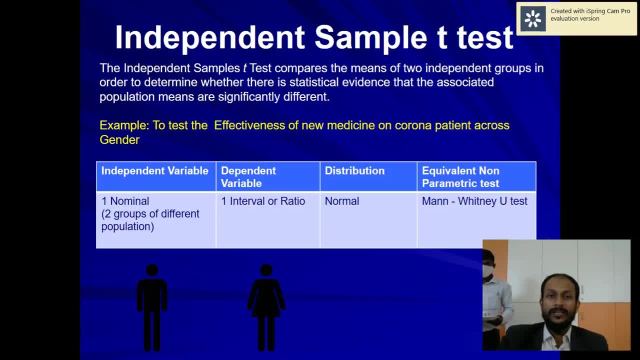 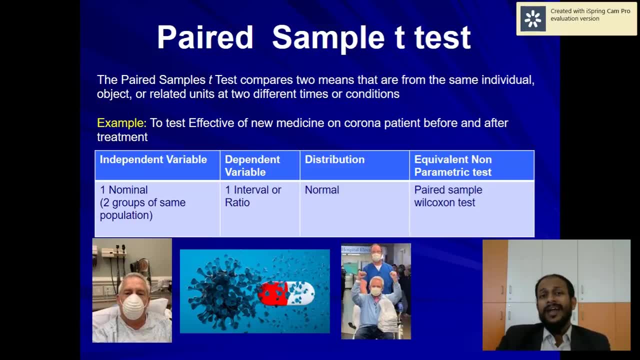 non-parametric test: man witness u-test. okay, fine, let us discuss about the pad sample t-test, the other technique now. here in pad sample t-test we compare the means of the same population. look at the difference between independent sample t-test and pad sample t-test. in independent, 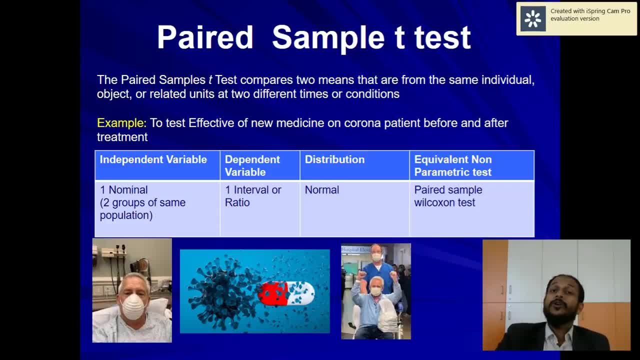 sample t-test, i am comparing the means across two different population. in pad sample t-test i am comparing the means across two samples of the same population. now let me explain it. say, for example: here also i am taking this corona as an example i wanted to have. i am. 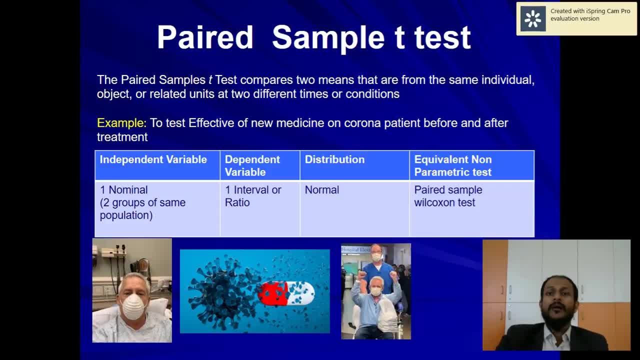 checking the new medicine of corona across patient before and after the treatment. now, most of the time i use this pad sample t-test in terms of conditions or in terms of situation. that means the population will be same. say, for example, before this session, what was your knowledge on data analysis? what is going to? 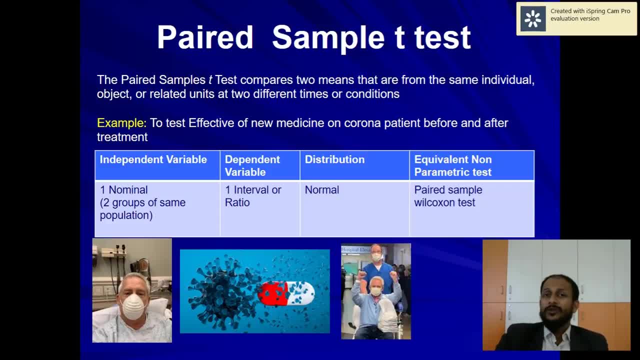 be your knowledge on data analysis, if at all. i wanted to use this assessment and the type of test. what i will be using is pad sample t-test. in this case, i am giving the medicine, i am giving the treatment, i am checking what was their body temperature before the treatment. 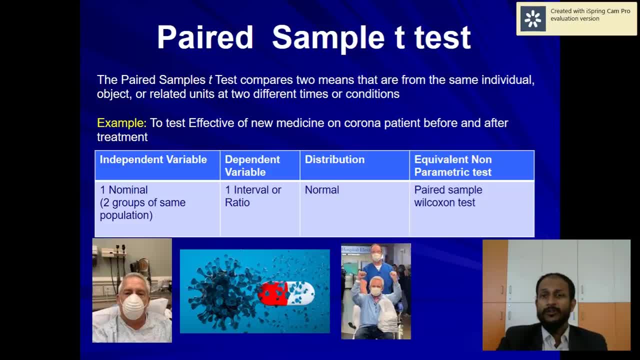 That means the population will be same. Say, for example, before this session, what was your knowledge on data analysis? What is going to be your knowledge on data analysis, If at all? I wanted to use this assessment and the type of test. 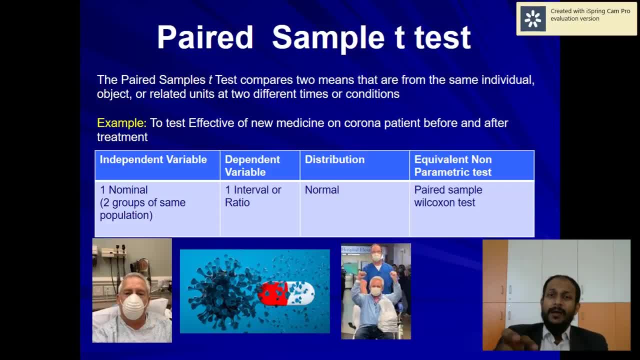 what I'll be using is pad sample t-test. In this case, I'm giving the medicine, I'm giving the treatment. I'm checking what was their body temperature Before the treatment and what is their body temperature after the treatment Across the same patient, not with different people, unlike independent sample t-test. 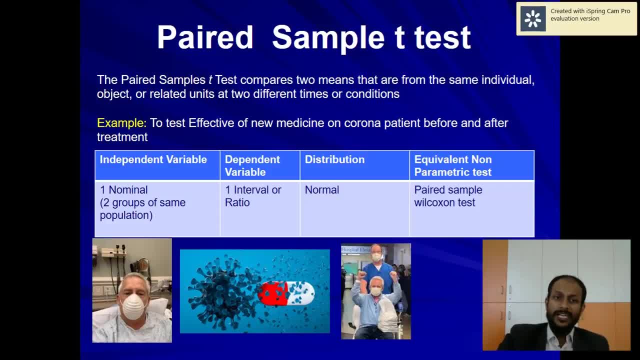 Now, when I'm using this technique is what I call it as pad sample t-test, And I have also mentioned the characteristics of the scale that independent variable will need to have and dependent variable need to have, And I have also mentioned the equivalent non-parametric test which we will be using. 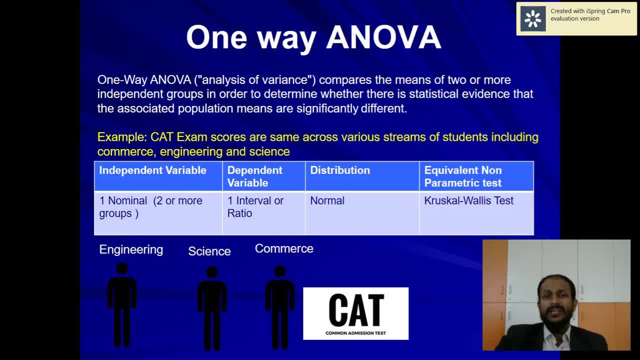 the technique called pad sample wilcoxon test. Now let us discuss about the one way ANOVA. What do you mean by this one way ANOVA? Here, also here I compare the means of not just only two population, but two or more population. 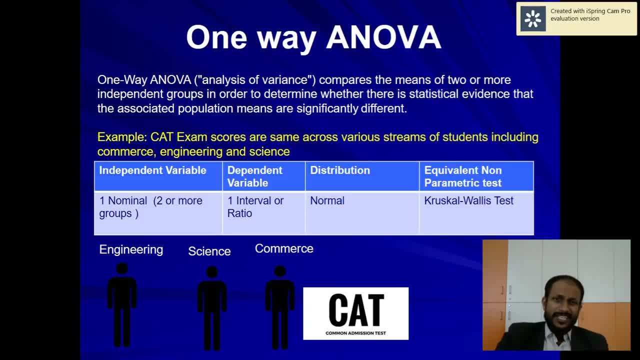 Now. so this ANOVA and t-test- both these tests- I use it for comparing the means. When I'm comparing the means across two population, I will be using t-test. In ANOVA, I can compare the means across two population, that is, two groups of population or two or more groups of. 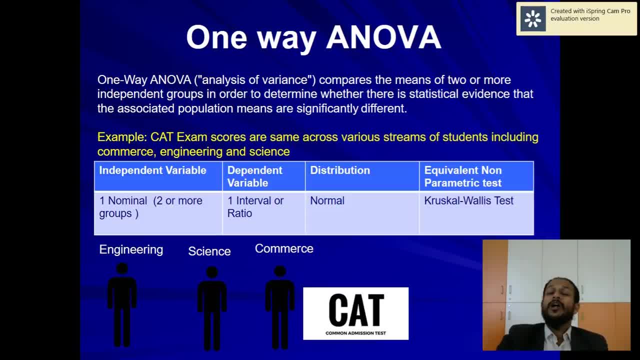 population, but typically I will be using one-way ANOVA to compare three or more groups of population. why, though, I can compare two groups? this the study says that student t-test is more powerful than ANOVA test when it comes to comparing two groups, so when I wanted to compare two group, I prefer to go for 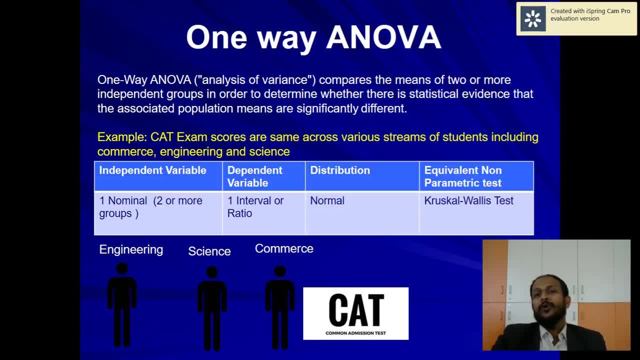 student t-test. but when it comes to three or more group, I prefer to go for ANOVA. when it comes to one-way ANOVA, in this case I am comparing the means of two or more group, but I will be having only one independent variable. now I will 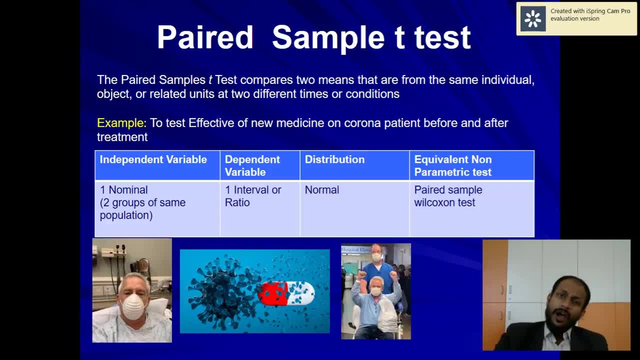 and what is their body temperature after the treatment across the same patient. okay, not with different, different people, unlike independent sample t-test. now, when i'm using this technique is what i call it as pad sample t-test, and i have also mentioned the characteristics of the scale that independent variable need to have. 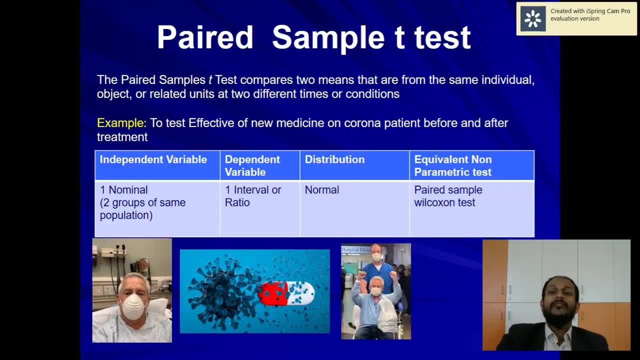 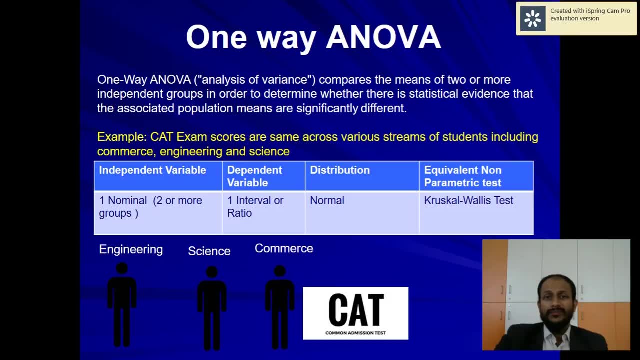 and dependent variable need to have, and i have also mentioned the equivalent non-parametric test, which we will be using, a technique called pad sample wilcoxon test. now let us discuss about the one-way ANOVA. what do you mean by this one-way ANOVA? here, also here, i compare the means of not 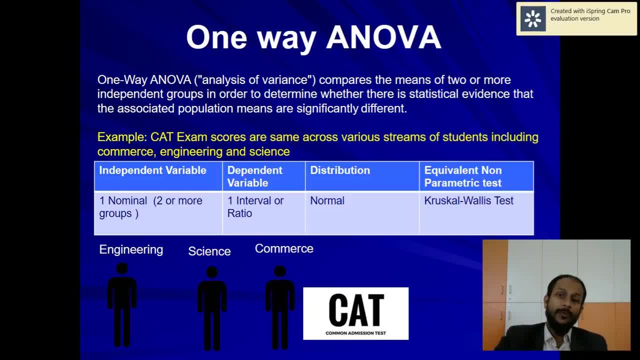 just only two population, but two or more population now. so this ANOVA and t-test- both these tests- i use it for comparing the means, when i'm comparing the means across two population. i will be using t-test in ANOVA and t-test- both these tests. i use it for comparing the means, when i'm comparing the. 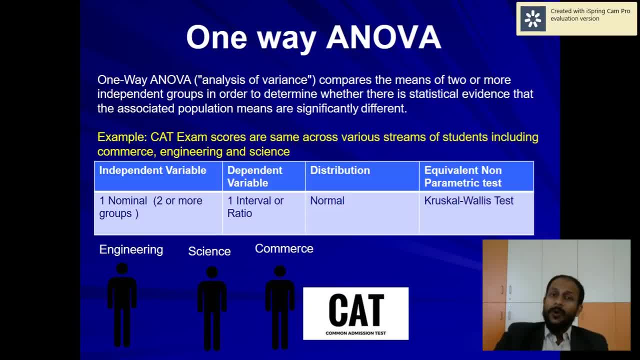 ANOVA, i can compare the means across two population, that is, two groups of population or two or more groups of population, but typically i will be using one-way ANOVA to compare three or more groups of population. why, though, i can compare two groups? this: the study says that. 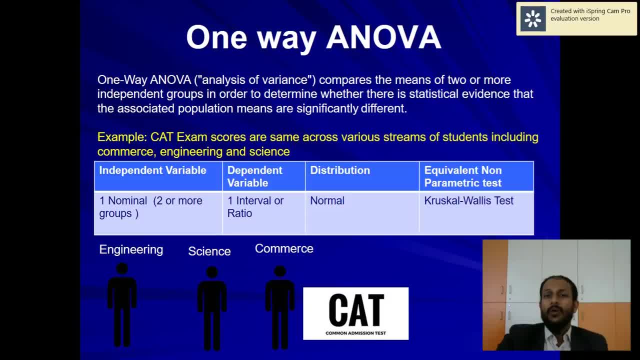 student t-test is more powerful than ANOVA test when it comes to comparing two groups. so when i wanted to compare two group, i prefer to go for two groups, and when i wanted to compare two groups for student t-test, but when it comes to three or more group, i prefer to go for ANOVA. when it comes 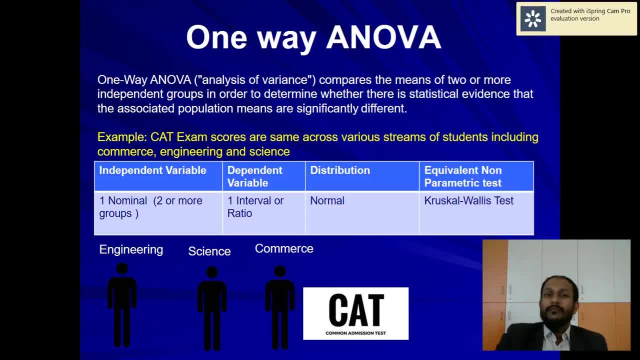 to one-way ANOVA. in this case i am comparing the means of two or more group, but i will be having only one independent variable. now i will be explaining it further when we talk about two-way ANOVA, so that we will compare two-way ANOVA with one-way ANOVA. i'll give you an example. let's say: 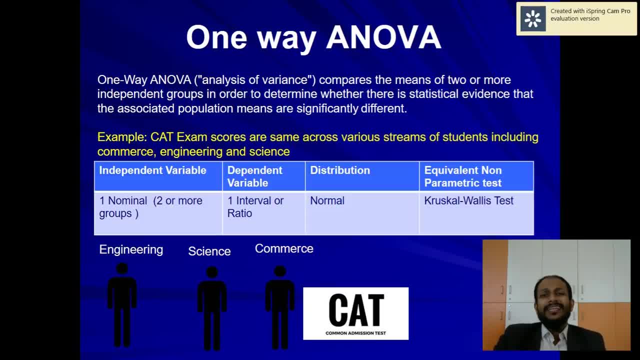 for example, that we are comparing the cat cat test exam scores across the various streams of students, including commerce, engineering and science. when i am doing this type of comparison, the kind of test what i will be using is ANOVA, because cat score is a dependent variable and different streams or three different groups. okay, 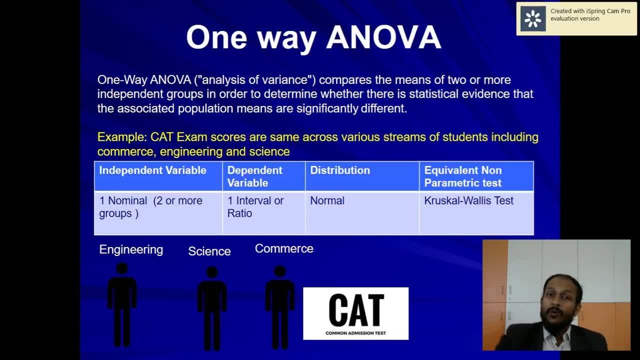 be explaining it further when you talk about two-way ANOVA, so that we will compare two-way ANOVA with one-way ANOVA, I'll give you an example. let's say, for example, that we are comparing the cat- cat the cat test exam scores across the various streams of students, including. 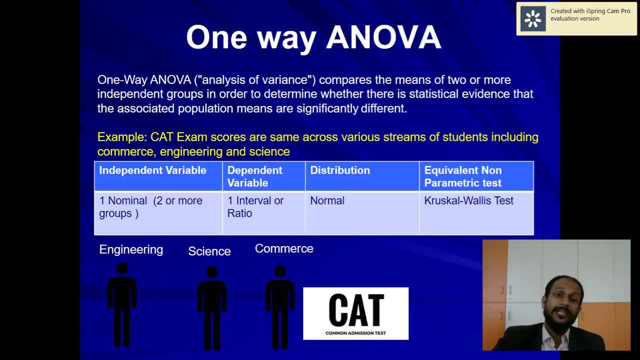 commerce, engineering and science. when I am doing this type of comparison, the kind of test what I will be using is ANOVA, because cat score is a dependent variable and different streams or three different groups, okay, so the perfectly I can use one-way ANOVA for this example. equivalent non-parametric test I can use. 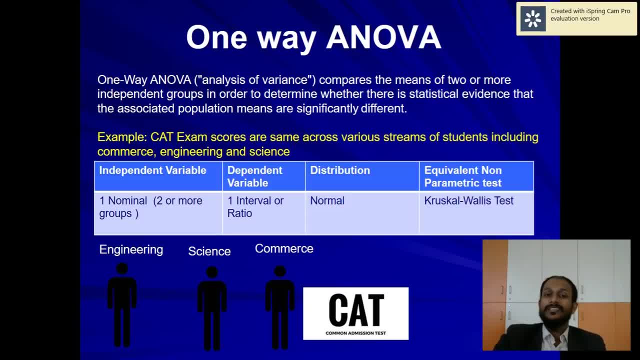 a test like Kruskal-Vallis test, one-way ANOVA for this example, equivalent non-parametric test. I can use a test like Kruskal-Vallis test when it comes to this scenario. so mean when we are comparing across three or more groups of population. that time I 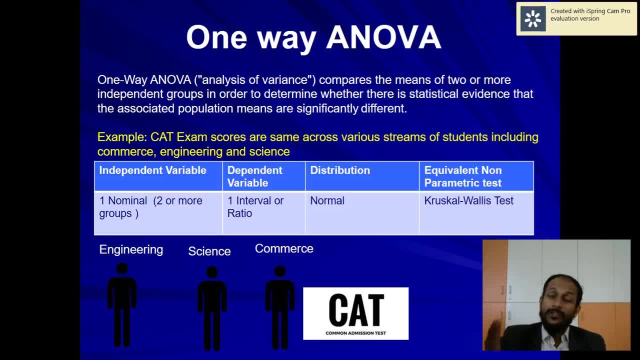 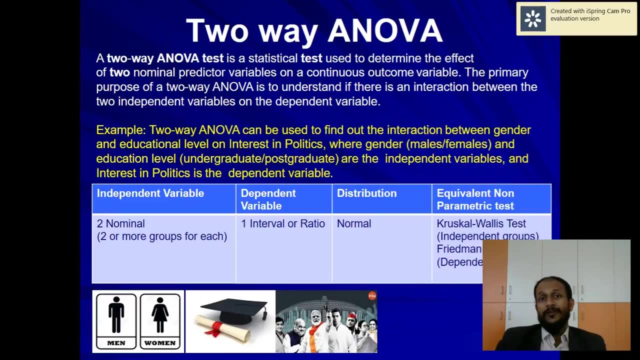 will be using a test called one-way ANOVA, though it is also capable of testing two groups. I prefer to use student t-test over one-way ANOVA when it comes to two groups, more than two groups, I go for one-way ANOVA now. when it comes to two way ANOVA, here is the difference now. Now, in one-way ANOVA, I was actually having only one test type, which means that I am having only one test type. how many inputs issues I would have, unless these tests are testing operations and increase quality, and when it comes to consume weight in number, two points. now, when it comes to two-way ANOVA, here is the difference. now, in one way ANOVA, I was actually high. 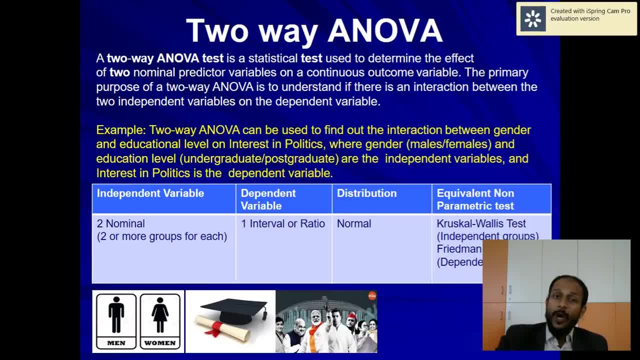 nominal variable and one interval variable. under one nominal variable i had two groups. but when it comes to 2a ANOVA, here i am having two nominal variable with two groups each and one interval variable and normal. now in this case i will be using 2a ANOVA. that means if the application is. 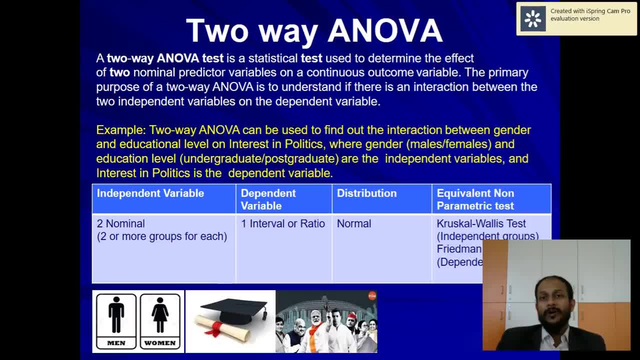 same. but instead of i having one nominal variable for independent in case, if i have two nominal variable with, of course, different subgroups, that time i will be using 2a ANOVA. but what is the application of 2a ANOVA? when will i use 2a ANOVA? basically, i am using 2a ANOVA just to. 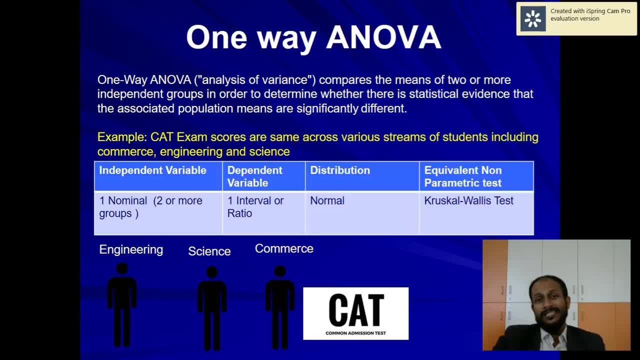 so the perfectly. i can use one-way ANOVA for this example, equivalent non-parametric test. i can use a test like Kruskal-Vallis test, which is a non-parametric test, which is a non-parametric test when it comes to this scenario. so mean when you are comparing across three or more groups of 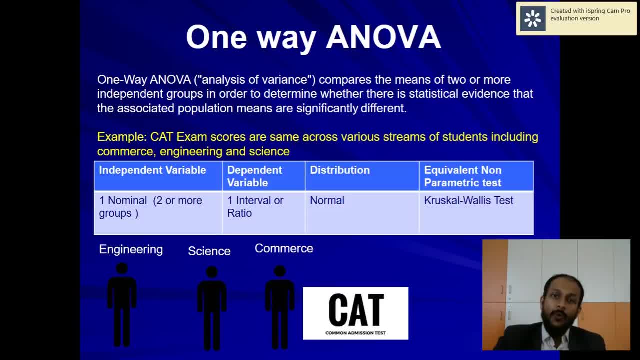 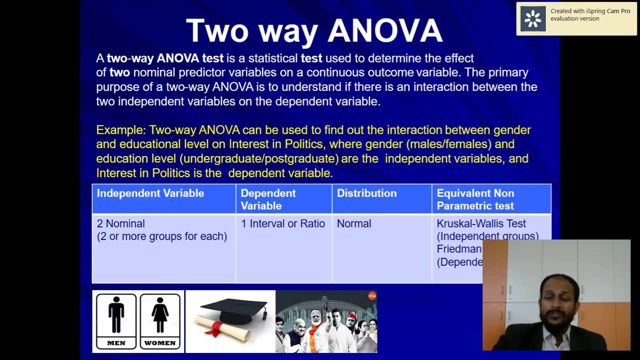 population. that time i will be using a test called one-way ANOVA, though it is also capable of testing two groups. i prefer to use student t-test over one-way ANOVA. when it comes to two groups, more than two groups, i go for one-way ANOVA. now, when it comes to two-way ANOVA, here is the. 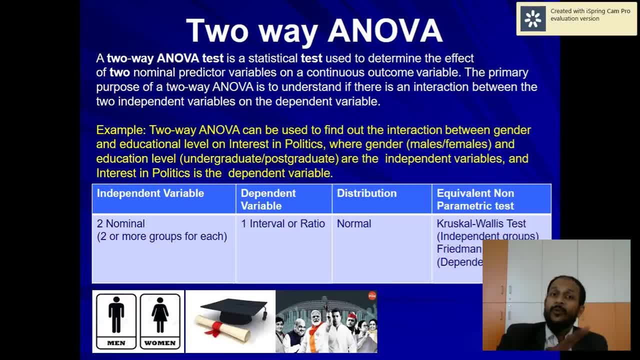 difference now. in one-way ANOVA i was actually having only one nominal variable and one interval variable. under one nominal variable i had two groups. but when it comes to two-way ANOVA, here i am having two nominal variable with two groups each and one interval variable and normal. now in this case i will be using two-way ANOVA. that means 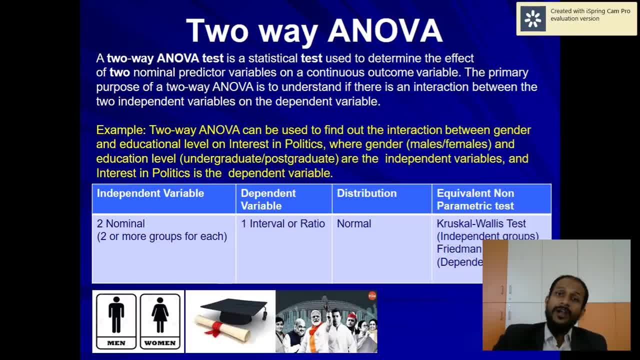 if the application is same. but instead of i having one nominal variable for independent in case, if i have two nominal variable with, of course, different subgroups, that time i will be using two-way ANOVA. but what is the application of two-way ANOVA? when will i? 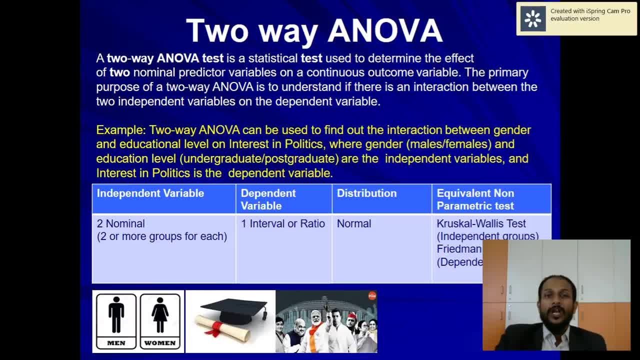 use two-way ANOVA. basically, i am using two-way ANOVA just to determine the effect of both the two nominal variables on the dependent variable, or, in other words, when i wanted to find out the interaction effect of independent variable on the dependent variable. only that case i will be using. 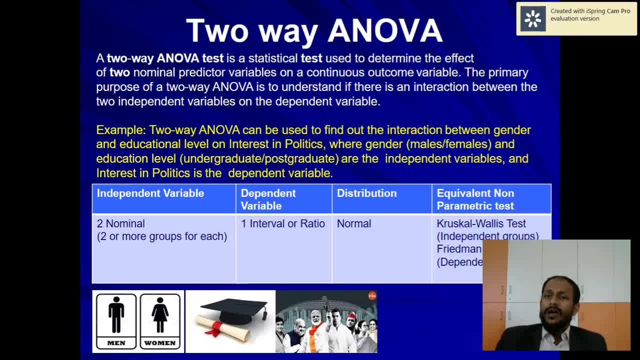 this two-way ANOVA technique. let us say that i wanted to start to study the interaction effect of gender and educational level with interest to politics. let's say that i am collecting whether a person is interested in politics in the rating of 0 to 100. 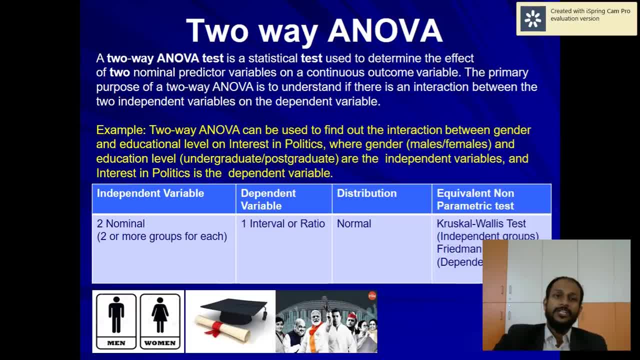 okay, that is. it may be either in interval scale or it is in ratio scale and i check it out whether somebody is male or female. and i am also asking one more question: what is his or her qualification? 10th, 12th, ug and pg, whatever it is now i am actually finding 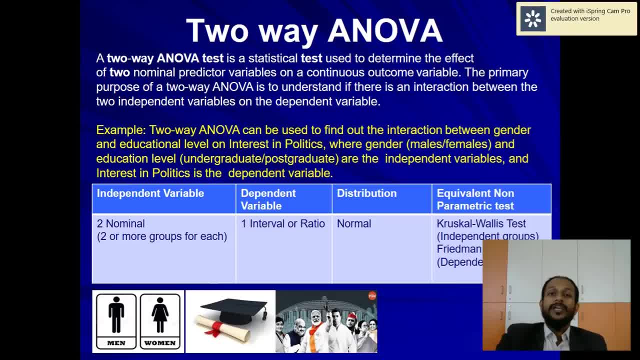 determine the effect of both the two nominal variables on the dependent variable, or, in other words, when i wanted to find out the interaction effect of independent variable on the dependent variable. only that case i will be using this 2a ANOVA technique. let us say that i wanted to study the interaction effect of gender and educational 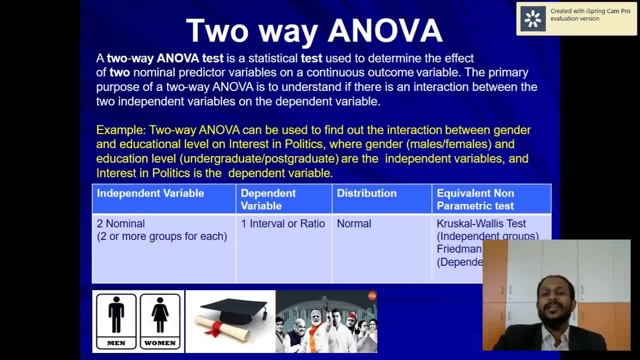 level with interest to politics. let's say that i am collecting whether a person is interested in politics in the rating of 0 to 100. okay, that is. it may be either in interval scale or it is in ratio scale, and i check it out whether somebody is male or female. and i am also asking one more: 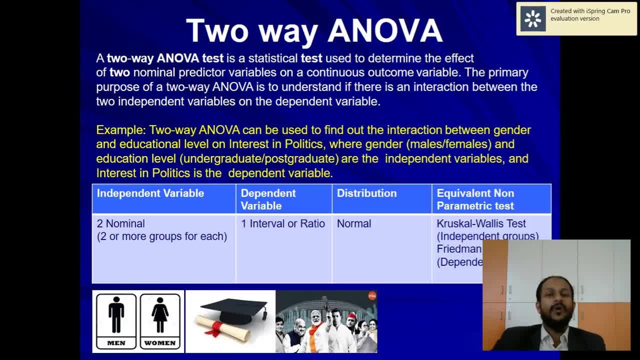 question: what is his or her qualification? 10th, 12th, ug and pg, whatever it is? now i am actually finding out the combined effect, the interaction effect of gender or politics, and how this relationship is being affected by a third variable called this one, whether it is a undergraduate or postgraduate, or it could be vice versa. here i 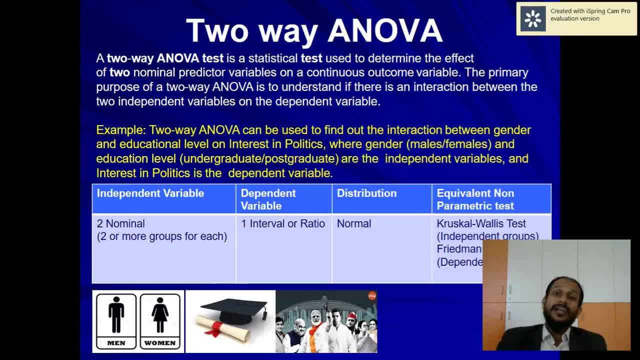 wanted to find out how the education level is affecting the interest in politics and how it has been influenced by gender. so now, let us understand: the strength of the impact of education level on interest in indian politics is affected by the gender. so now, this is what we call it as interaction. 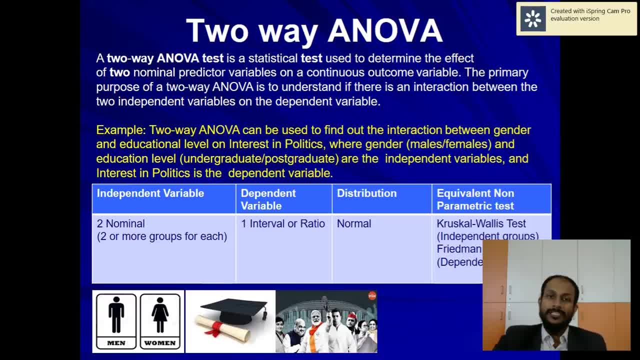 effect this. we have explained it further in the previous videos which you can always refer. so if this is your situation, you can use something called 2-way ANOVA provider. it fulfills the assumptions of parametric test. if it is not fulfilling any of the assumptions of parametric, 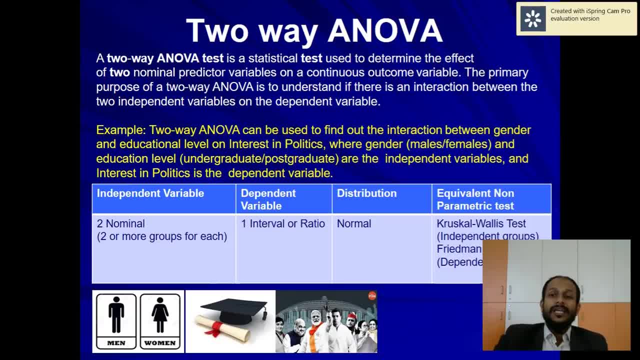 test that we have already discussed, then, not to worry about it, we have an equivalent test called either Kruskal valleys test, in case, if you are using independent group. otherwise you can use Friedman test if, in case, you are using a dependent test, dependent groups, right? the last one is about 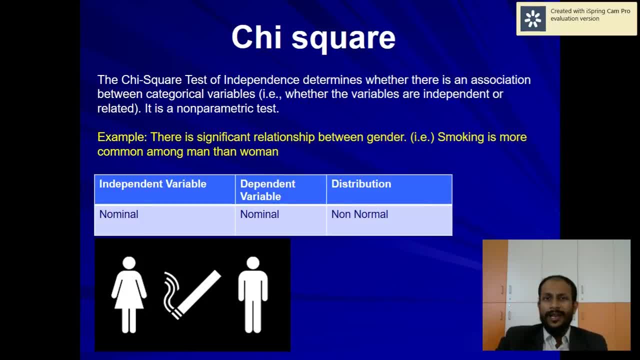 the chi-square test. nothing to complicate it because it is not a parametric test, so naturally there is no assumptions of normality. you may not worry about the fulfilling the other assumptions of parametric tests, like I have discussed. but this is also a very popular technique which 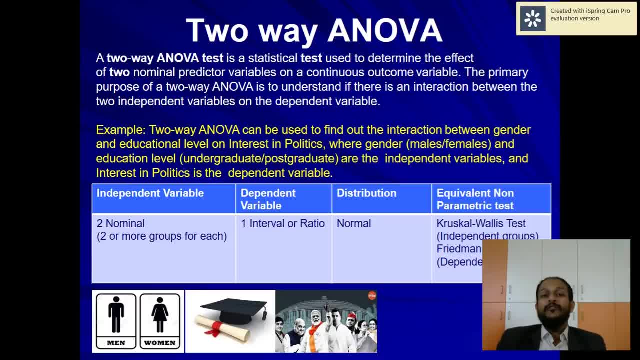 out the combined effect, the interaction effect of gender on politics, and how this relationship is been affected by a third variable called this one, whether it is a undergraduate or postgraduate, or it could be vice versa. here i wanted to find out how the education level is affecting the interest in politics and how 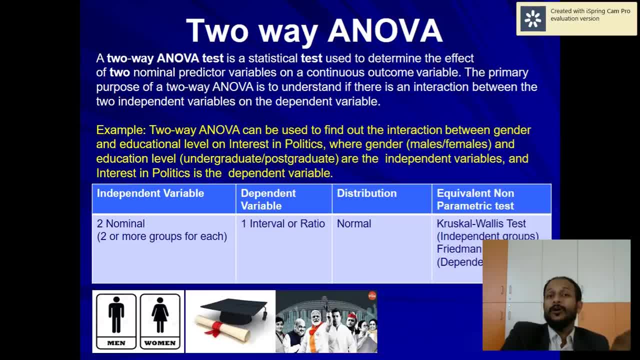 it has been influenced. the strength of the impact of education level on interest in indian politics is affected by the gender. so now this is what we call it as interaction effect. this we have explained it further in the previous videos which you can always refer. so if this is your situation, you can use something called two-way ANOVA. 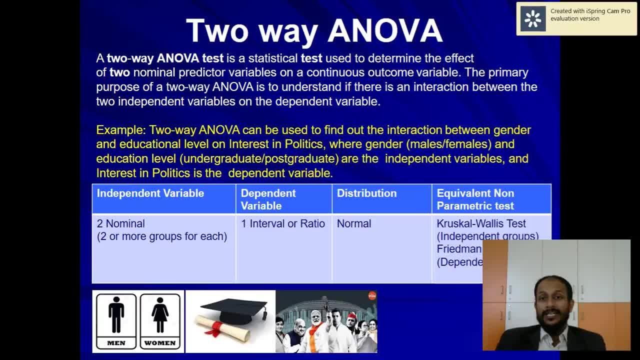 provider it fulfills the assumptions of parametric test. if it is not fulfilling any of the assumptions of parametric test that we have already discussed, then not to worry about it. we have an equivalent test called either Kruskal valleys test, in case if you are using independent group. otherwise you can use Friedman test if, in case, you are using a. 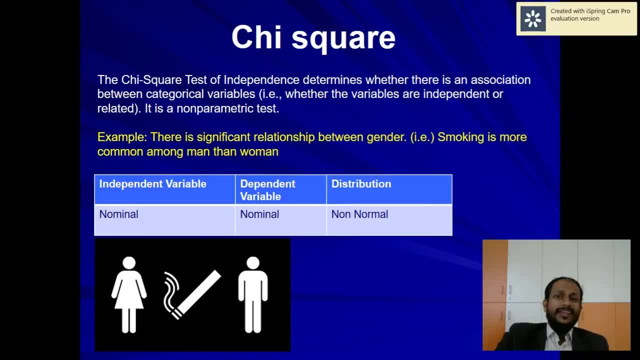 dependent test: dependent groups: right. the last one is about the chi-square test. nothing to complicate it because it is not a parametric test, so naturally there is no assumptions of normality. you may not worry about the fulfilling the other assumptions of parametric test, like i have. 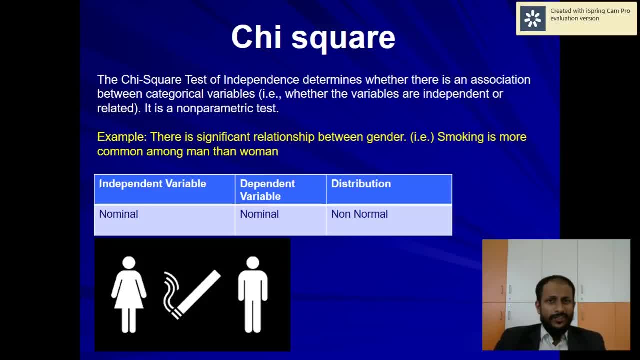 discussed. but this is also a very popular technique which researchers uses, because here both the independent and dependent variable, both the scales, are nominal. okay, they are not any continuous scale. let's say that you wanted to study the relationship between gender and smoking and you think that the smoking is more among men than women. 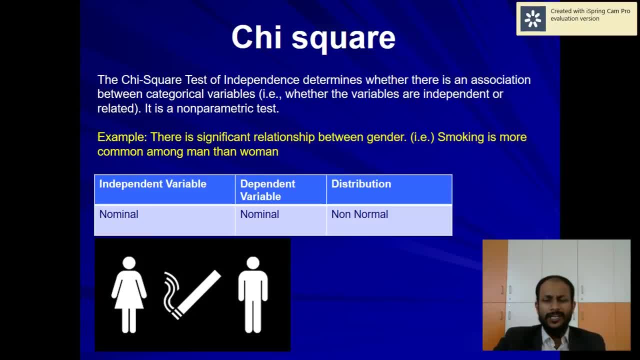 so now, how do you do that? you ask two questions, please indicate your gender, and you ask a second question, whether you smoke or not. so now, what do you do? you perform a simple test called chi-square test, which has a cross tabulation, and you find it out whether this smoking and gender is it. 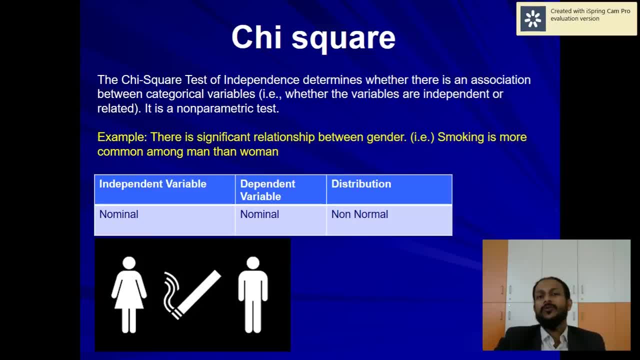 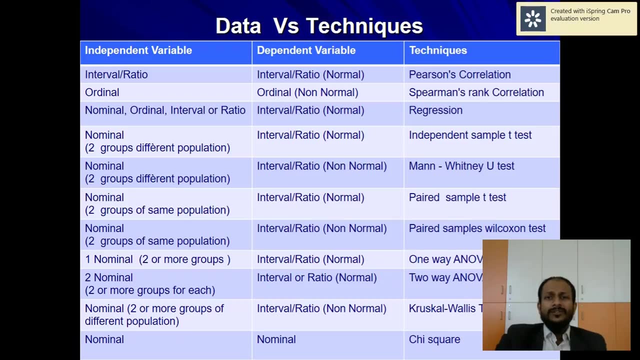 interrelated with each other and the kind of test, what you will be using in this case would be chi square test. okay, and there is not mandatory that you need to have a kind of normal distribution curve for this, because it is both of them are nominal datas, right? so now what i'm trying to. 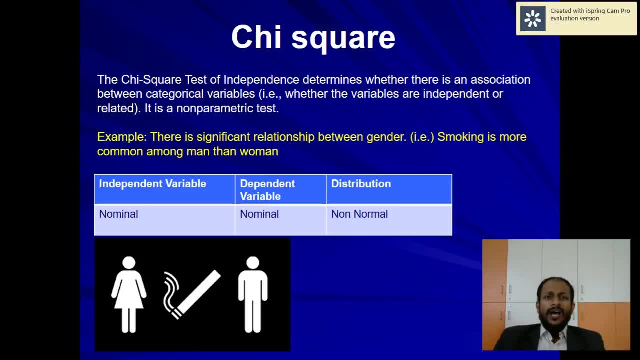 researchers uses, because here both the independent and dependent variable, both the scales are nominal. okay, they are not any continuous scale. let's say that you wanted to study the relationship between gender and smoking and think that the smoking is more among men than women. also, now, how do you do that? you ask two questions. please indicate your gender and you ask: 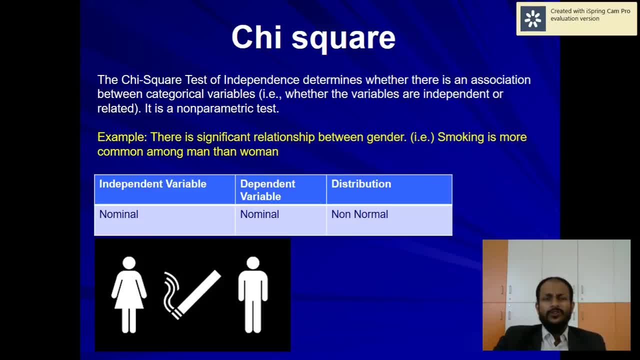 a second question: whether you smoke or not. so now, what do you do? you perform a simple test called chi-square test, which has a cross tabulation, and you find it out whether this smoking and gender- is it interrelated with each other? and the kind of test, what you will be using. 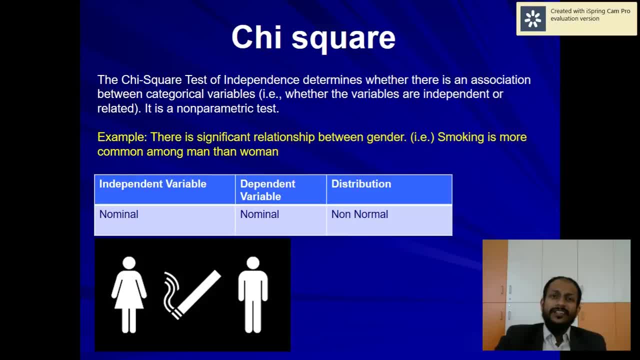 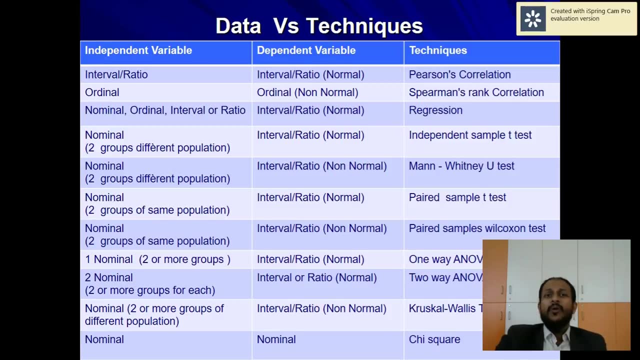 in this case would be chi-square test. okay, and there is not mandatory that you need to have a kind of normal distribution curve for this, because it is both of them are nominal datas, right. so now, what I'm trying to say is this one: now, if you can see this slide, I have clearly mentioned 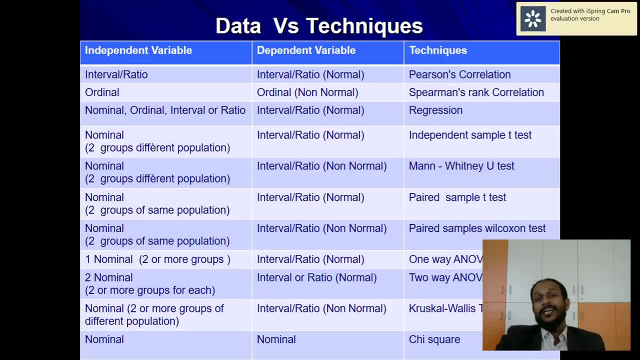 what type of data and what type of technique that I can use. it. very clearly, you can take a screenshot of it, I don't mind, so that it becomes a quick reference for you to find it out what type of test that I can use for what type of application. right, so let me conclude this session. 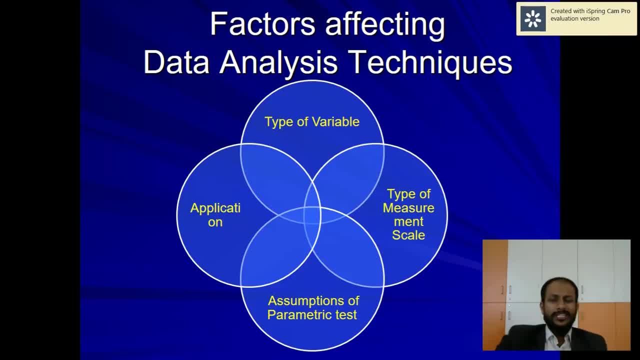 a very long session by a small note. now, what I'm trying to say is that refer to the previous two videos and kindly recollect the video that we have discussed it today. when it comes to the right data analysis technique, it has been affected by four important things. first, what is the kind of 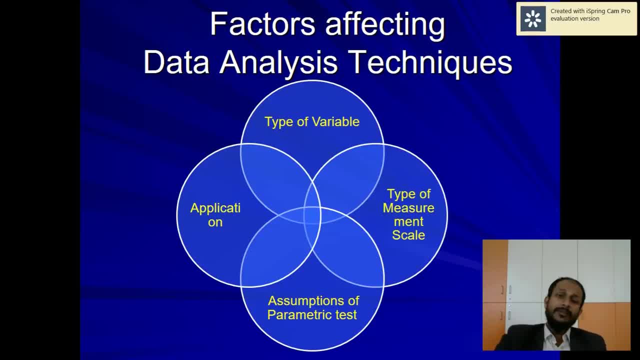 variable that I have, that I have identified. is it an independent variable, dependent variable? is it a mediating variable, moderating variable? that we have to check it out, number one. number two is that: what is the type of measurement scale I have? is it a nominal, ordinal? 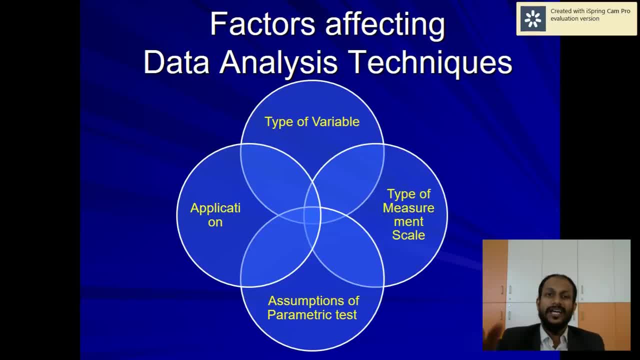 ratio or interval. no, that is one side. and third one is that is my data fulfilling the assumptions of parametric test, those six or seven assumptions that I have already mentioned? you can refer it out. and fourth one is that: what is the application? what is the situation? so, based on these four,